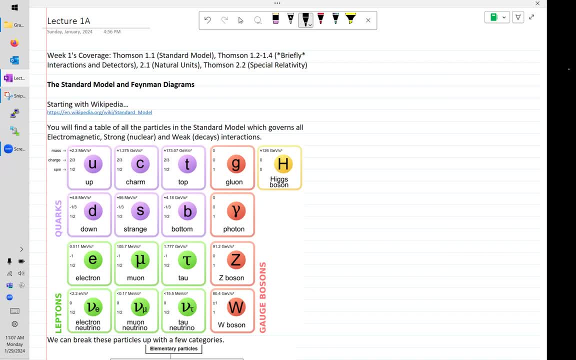 And we'll see how far we can get on special relativity, because I think I'm I'm slating us on a lot on the plate and then see how far we get. So we may have to cover special relative beginning next week anyway. 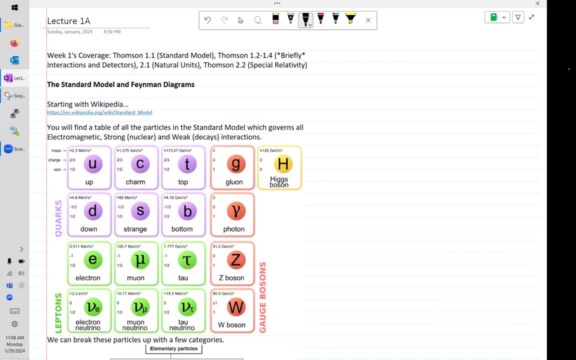 Okay, so the first section is on the standard model, and the standard model covers- as I think I tried to hint this last week- is that it covers three out of the four fundamental forces that we know about, and that's electricity, magnetism, which is combined together. 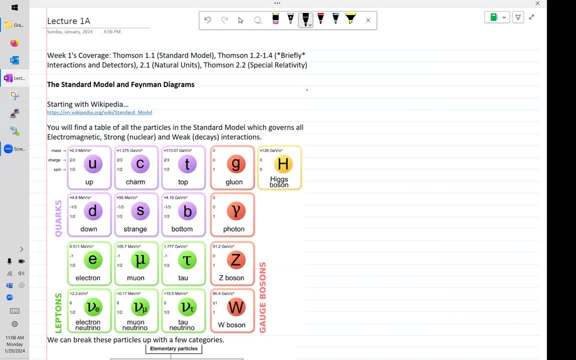 And that's electricity magnetism which is combined together. And that's electricity magnetism which is combined together. Those of you who took general physics from me will probably know why they are basically the same, because whether something is an electric field versus a magnetic field actually just depends on your frame of reference. 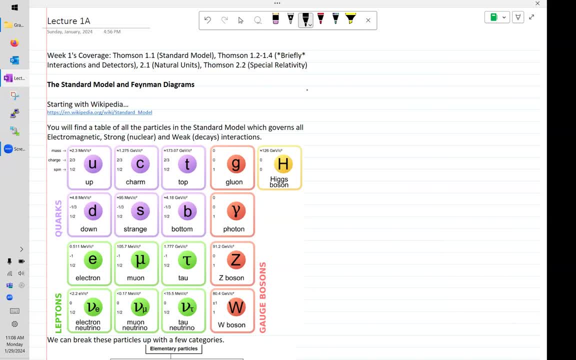 There's not a real difference. And then there's also the strong force, which is covered by electrochromodynamics and which is the stuff that binds nucleus and protons and neutrons together, And we're going to go through all these little particles in a little bit. 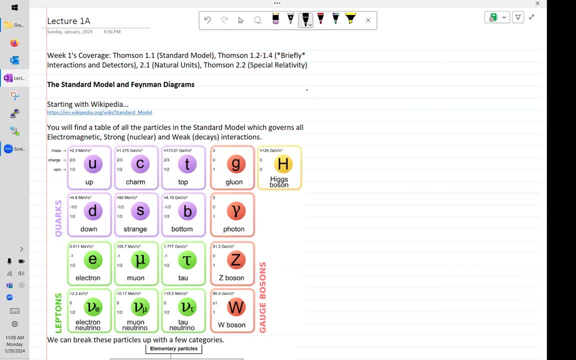 But the last one, The last one that we're going to cover is going to be the weak force, which you'll also see, is actually part of electromagnetic force. It will be combined with electricity and magnetism to make it an electroweak theory. 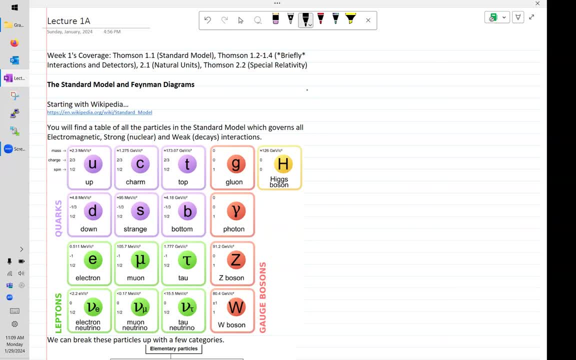 It will actually be merged together. And gravity we're not going to deal with. Okay, we don't deal with gravity in this class at all because we don't really have a standard model that describes it and do calculations with it, And that's covered in general relativity, which is a completely different way to think about how interaction and how things don't actually interact with each other. but it's just a space-time changing on you. 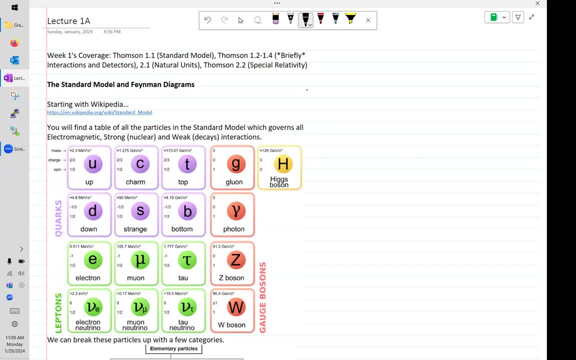 And that's a completely different type, And one of the ideas is that the hope is that at some point in the future all four of these forces can be combined together into a grand unified theory. That way we can cover everything under the The same mechanism. 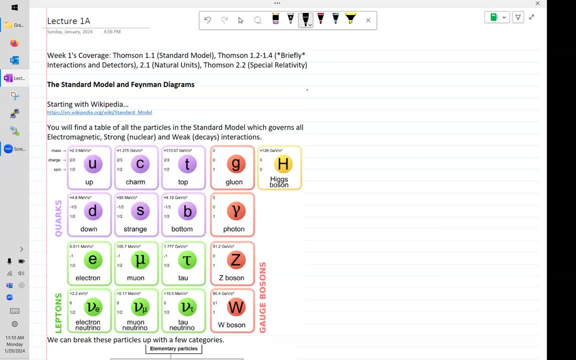 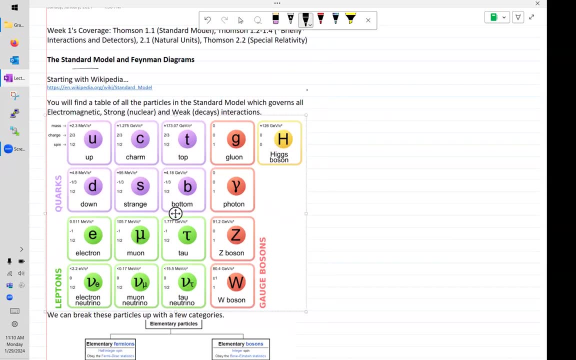 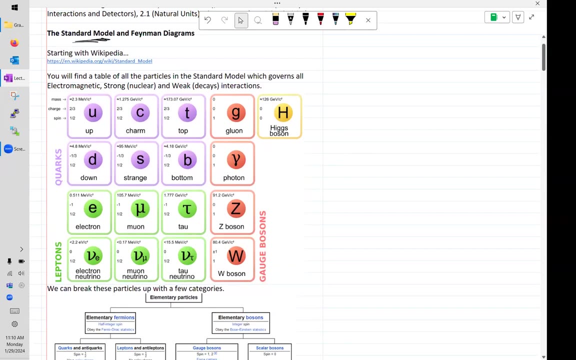 So we're not- you know, we don't have this- two different ways to make predictions and do calculations. Okay, So the first section here is going to be the standard model. Let's talk about what the standard model is. The standard model consists of these 17 particles. 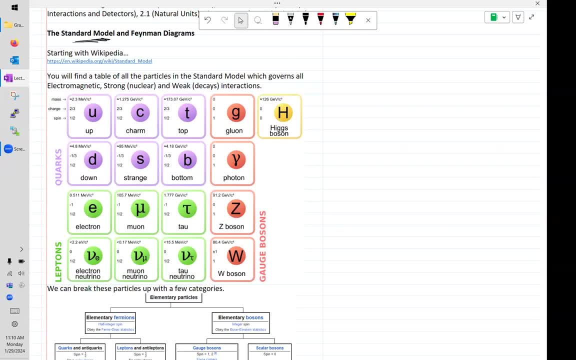 It's kind of nice that you don't have to memorize a lot of things, but there are these 17 things you have to get to know. Okay, So there are these things called quarks, which is, And this purple stuff, maybe pink depending on your screen. 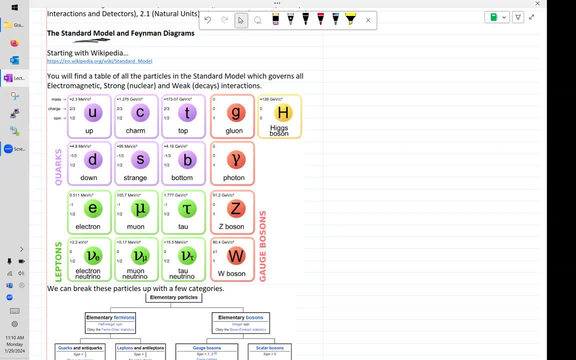 Okay, The quarks are actually what makes up protons and neutrons in everyday life. It can make other stuff also, and we'll talk about that, And most of the quarks that we see in everyday life is the up quark and the down quark. 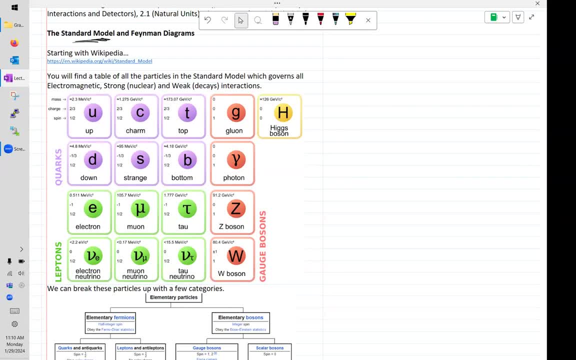 And it's very, you know, creative naming there, because it's just One, has a charge of two-thirds. I should just use the pen instead, So people can see me online. Let's do the red pen Right, Okay, And it has a spin of one-half. 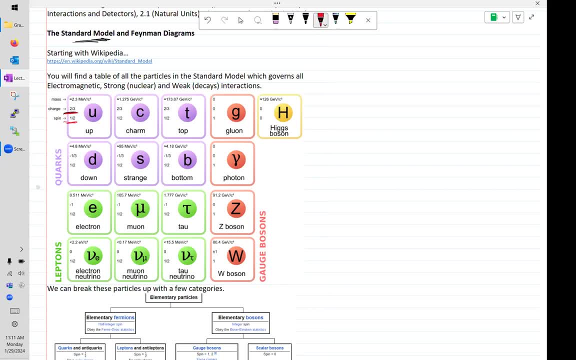 Okay, And we'll talk about what spins are and how does that correlate to how things are formed together? Okay, The down quark has an electric charge of one-third the electron charge. Okay, Remember the charge of an electron Q of E, right? 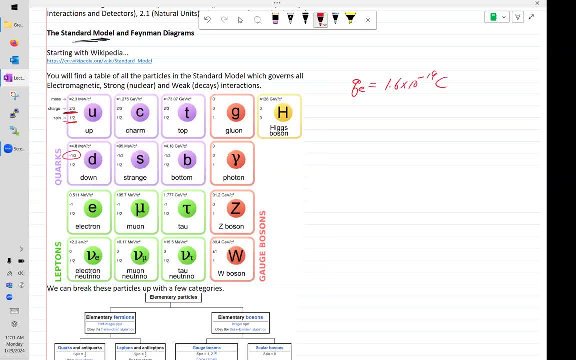 It's about 1.6.. It's about 1.6 times 10 to the negative 19 coulomb in this unit, and we'll get rid of this unit pretty soon because then we'll not have to deal with these conversion factors. 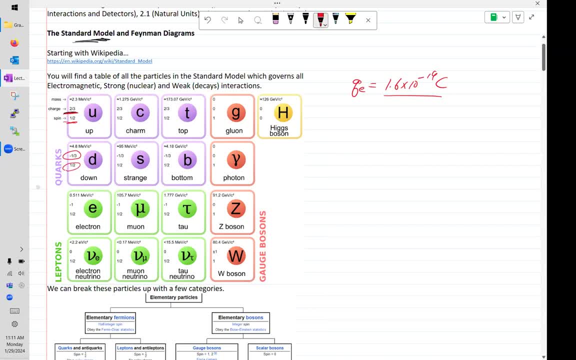 Okay, It also has a spin of one-half And when you have a proton, right a proton- I think the prior picture is down below somewhere- it's actually made up of two up quarks and one down quark, Okay. 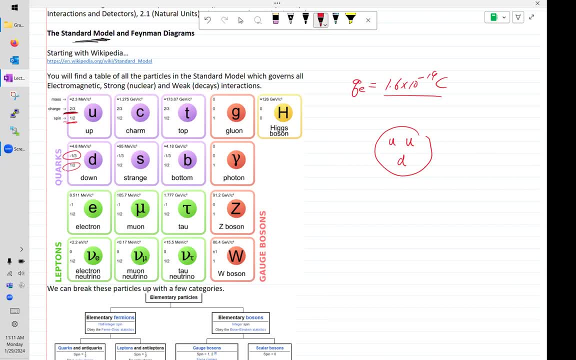 Right. And remember that the charge of a proton Right- This is actually the absolute value- It's the same as the charge of an electron Right, Also 1.6 times 10 to the negative, 19 coulomb Right. 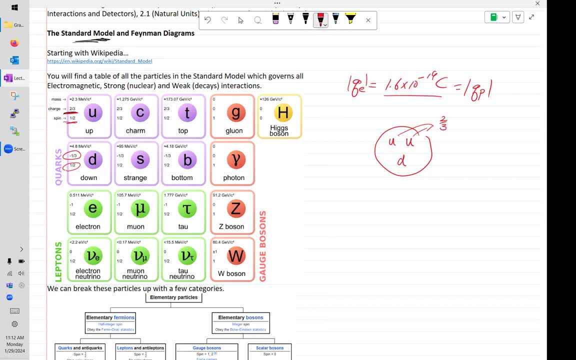 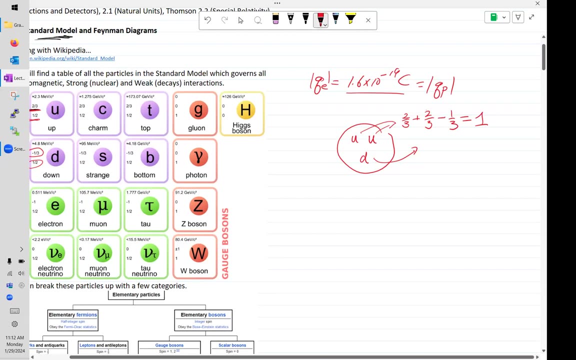 Since each of these up quarks has two-third right of the electric charge- fundamental charge right, the down quark has negative one-third Right. If you add all this up it adds up to exactly one Right. So the proton has the. 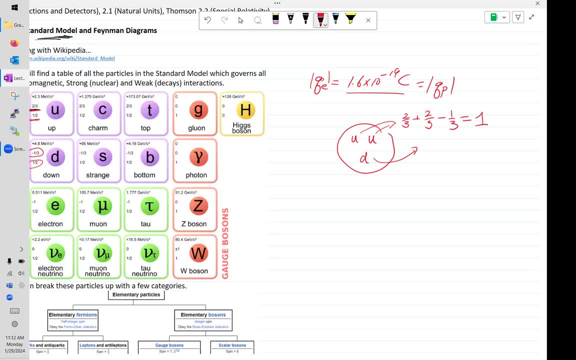 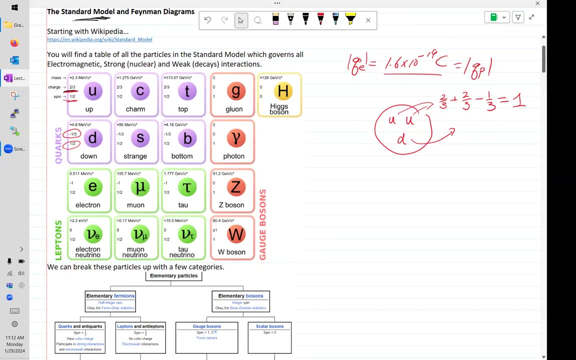 The same charge of an electron in magnitude right, because, right, it's made up of two up quarks and one down quark. Okay, Right, There are other generations of them. Okay, Meaning, there are like kind of like heavier version of them that we don't see every day. 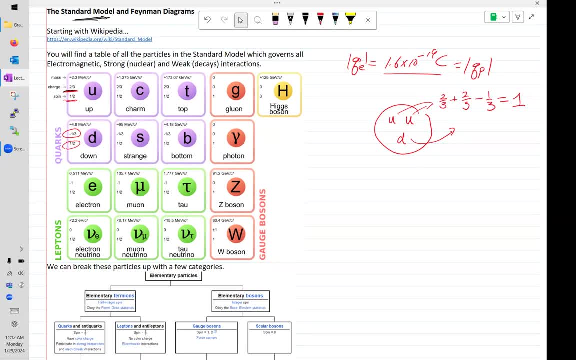 And usually these are produced in colliders and rare events and we don't deal with them in everyday life. But if you want to study them, you have to make them in these accelerators And stuff like that that we're going to talk about, hopefully tomorrow, on Wednesday. 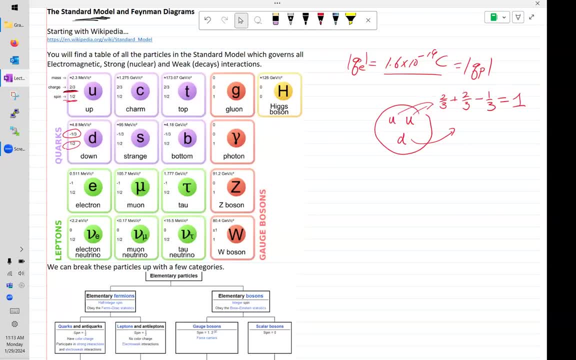 Okay, So the second generation for quarks is charm and strange. And then the third generation is top and bottom. I'm not going to go through the facts of these things, but the general trend is that the higher generation you go, the more massive they are. 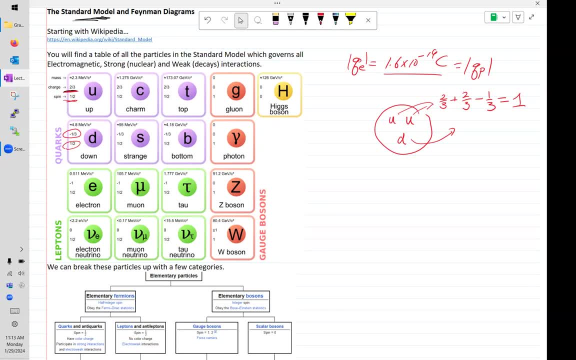 They're just like bigger and bigger and bigger. Okay, I don't want to say bigger and bigger, Heavier and heavier. Well, I don't want to say heavy, anyway. Also, heavy is like also a gravitational link thing. 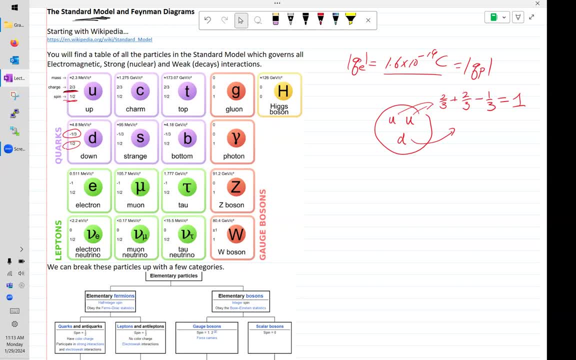 But more and more massive. Okay, All right, So that's the quark sector. And all of these right participate in the strong interaction. I'm going to see what these are, Okay, The weak interaction and the electromagnetic. I'm going to put EM here, if I can figure out my pen. 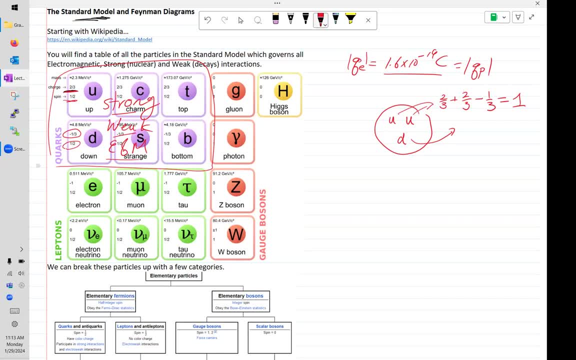 Okay, All three forces. Okay, All right, Okay, Okay. And the next thing down here are what's known as the leptons, the little green guys down at the bottom here. Okay, The leptons. So the leptons are a little bit different from the quarks because they do not interact with the strong force. 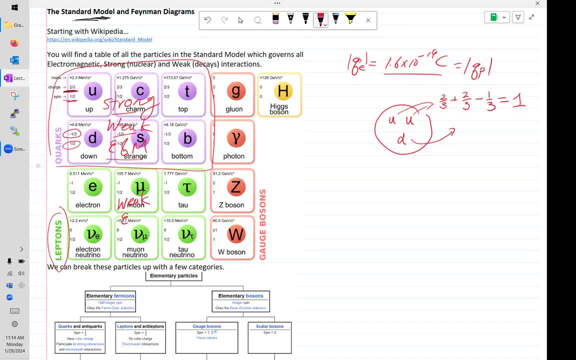 Okay, So just the weak. and well, make sure, I'm going to write EM on top, Electricity and magnetism on top, And then weak between the two And we're going to see why In a second. So hopefully you're. everyone's heard of an electron. 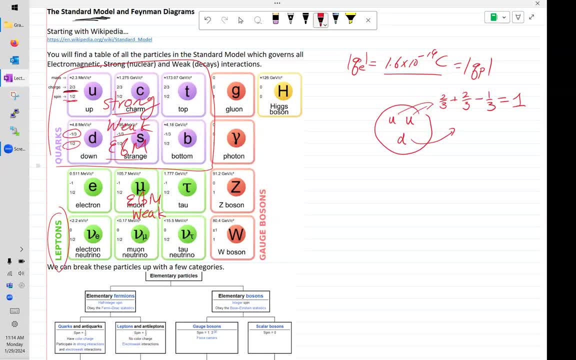 So electron is the lowest generation, lowest mass, lowest mass charge lepton. So this is a lepton that has a charge of negative one elementary charge right Negative. the charge on one electron is actually negative 1.6 times 10 to negative 19 coulomb. 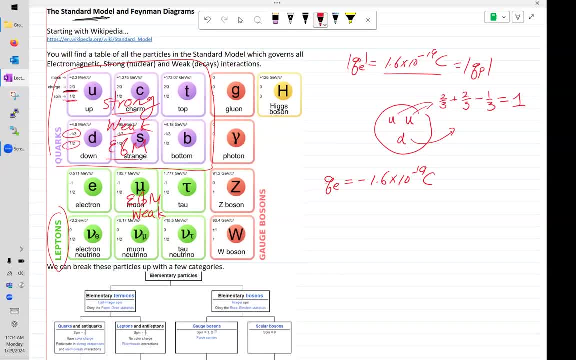 And this crazy units we used to. we use in general physics and intro physics to convert them to SI units. Okay, Before I go down here with the neutrinos, so there are also three generations of these leptons. right, So you have the electron. the next one up is called muon. 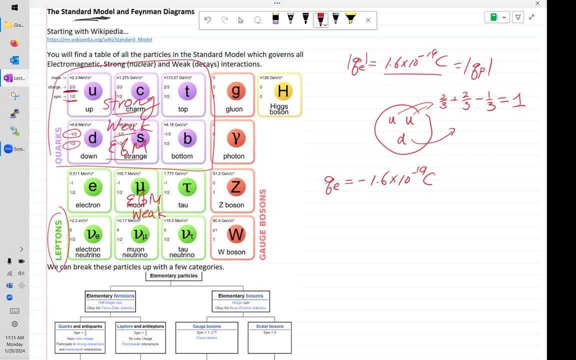 Okay, And there's some history about why it's called muon And then the next one is called tau. Yeah, Once again the same pattern happens where the electron is the lowest mass. So you can actually see the mass up here on the top left corner. 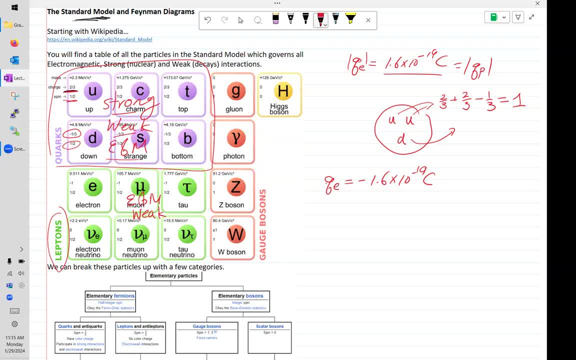 0.511 MeV Per second Per C square. So that's a unit of mass. So just think about them as just a number. Okay, Bigger number, bigger mass. We're going to figure out what these units mean a little bit. 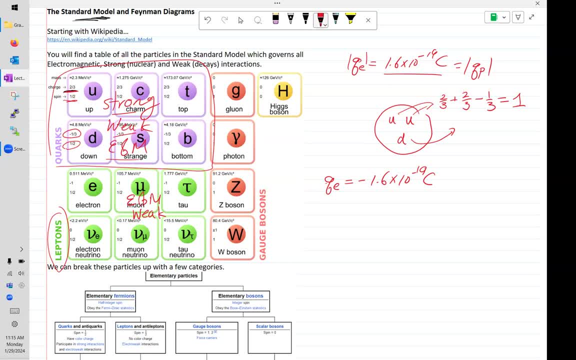 Okay, Okay, Where the muon is 106, the tau is actually 1,777, right, So it's actually about 3,500 times more massive than the electron, So it's like a really, really chunky electron. 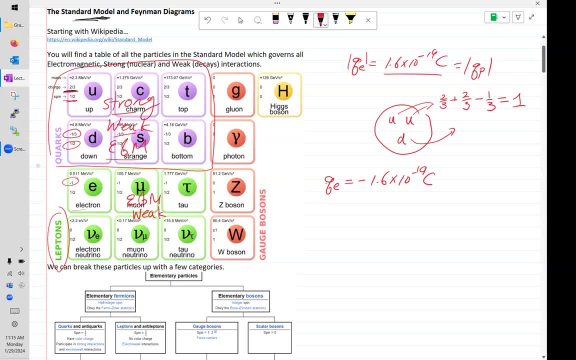 Okay, So all of these have electric charge and therefore they also interact with electricity in magnetism. Okay, So what happens is that? the difference is that, while the quark sector- well, all of them- have charges, right, Electric charges at least. 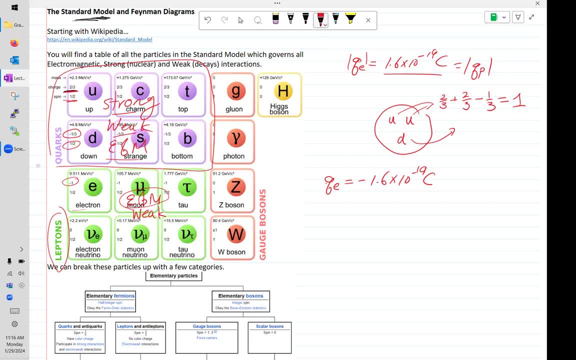 Okay, Where in the lepton sector there are those called neutrino, neutrino- the word neutrino hopefully dries up, you know. oh, something that's neutral, right, Okay, That means they do not have an electric charge. 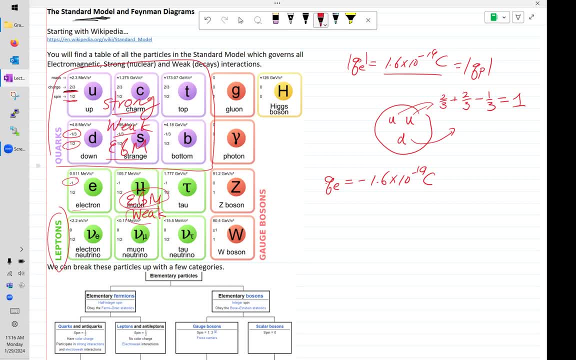 Okay, So there's no electric charge. The only thing they interact with is the weak force. Okay, So that's a big difference. Okay, So that's a big difference. Okay, And neutrinos are almost massless. In fact, before 1980s, people thought they were massless, and then people started measuring. 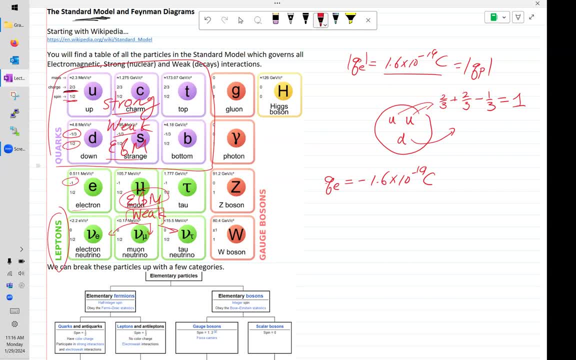 the this thing, this phenomenon called neutrino oscillation, And in order for them to oscillate into each other, you actually have to have mass, And but right as of right now, we are not able to measure the mass of these neutrinos. 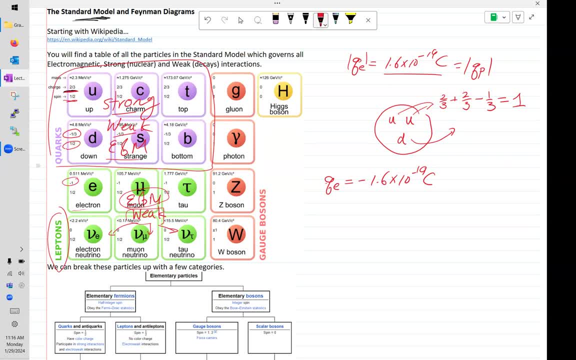 so far because they are so small. Okay, Just to give you guys a number. So so the top left corner here for the electron neutrino right, It's a less than 2.2 electron volts per C square. Okay. 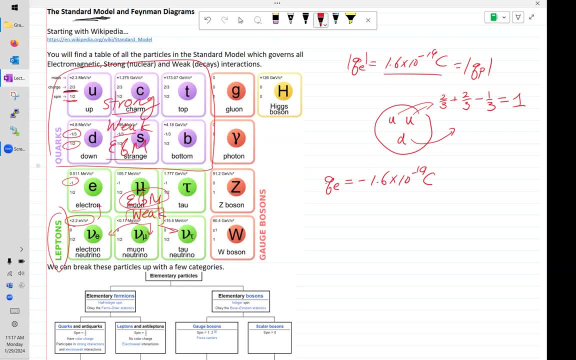 Compare that to the mass of an electron, which is 500,000 electron volts. So the mass of a neutrino is about 250 times, 250,000 times less than the mass of an electron, And electron's already very light right. 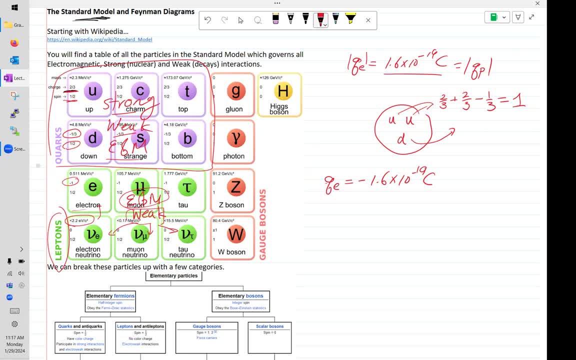 Okay, So this is why it's very difficult to measure these things, because they basically go at the speed of light whenever you put a little bit of energy into them And it's really difficult for us to determine what their mass is. Okay, Right. 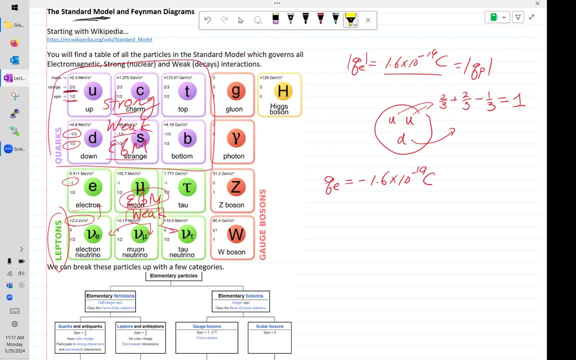 So the stuff on the left-hand side here, all this stuff over here, Whoa? Why does it give me a white screen? Okay, Nevermind. All of these things are called, also called fermions, And what does that mean? 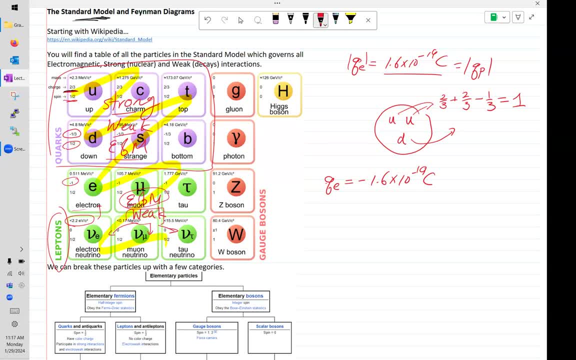 Okay, It means fermions And and, and. we're going to talk about what fermions are Okay, When we actually get to derive them Okay, But what's interesting is that all of the matter is always made up of these things. on. 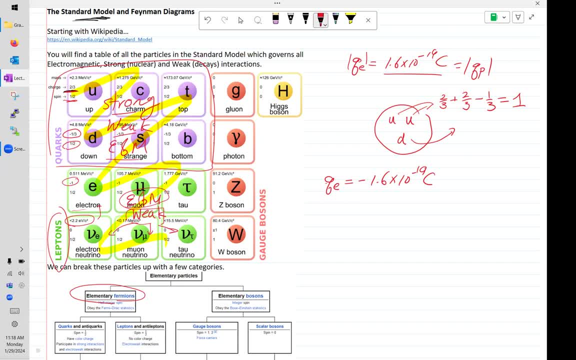 the left-hand side. Okay, The stuff on the right-hand side, or actually what's known as gauge boson, I'll just call them bosons. Okay, We don't need to add the gauge into them. Okay, I'm going to see what the difference between fermions and bosons is in a second down here. 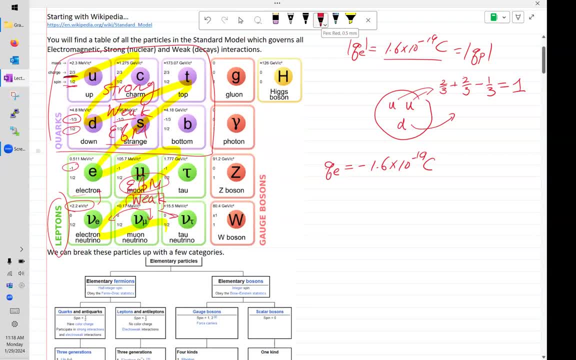 Right, But just to go back to the fermions, So notice that all of them have a spin of one half. Okay, And we're going to see what spin means. Okay, Fermions have spin of one half. Okay, The gauge bosons. 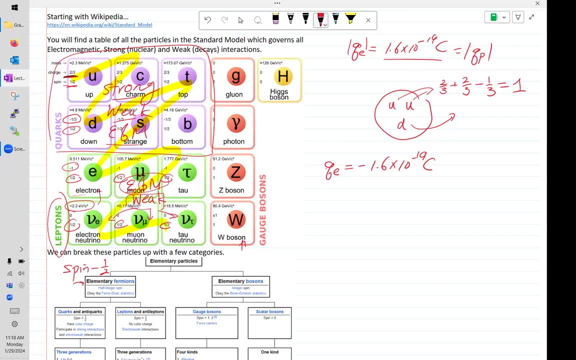 Okay, All of them will have the spin of one, Just one, Okay. Okay, And we'll see what that means. Okay, And we'll figure out what the spin things means. Okay, Because it's actually going to be useful in our calculation when we try and make predictions. 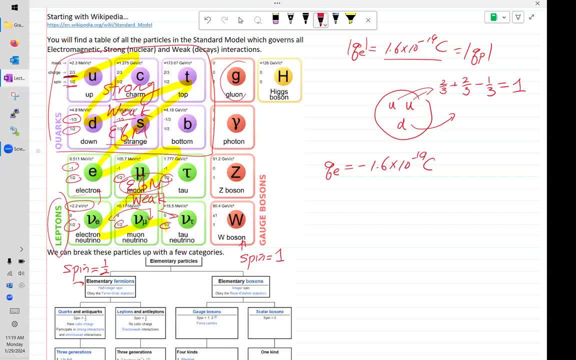 out of them. Okay, So there's the gluon, which is the strong boson. So you know that's the strongest one. So this guy is with the strong, Okay. Photons, hopefully, are familiar to most of you because, you can see, this is the electromagnetic. 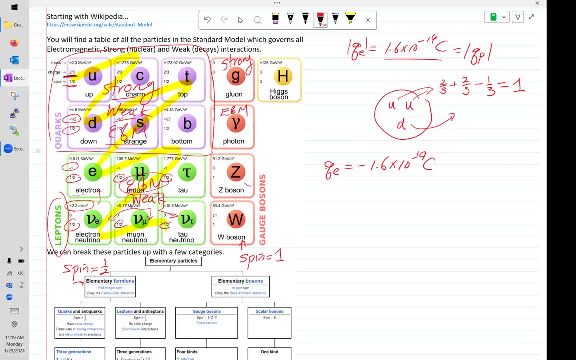 boson, Okay. And then the Z And the W. There's no names for them, Okay, They're just letters. Okay, These are the weak bosons. Okay, Sorry for the messiness. Okay, And when I was taking this class, basically that was it. 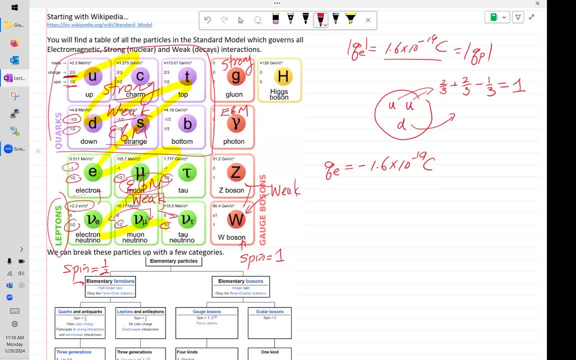 There was the 16 things together. Okay, Now that you're taking this class, past 2012,. we also- well, we knew the Higgs boson should be there, but we haven't confirmed it yet, So we're going to go ahead and do that. 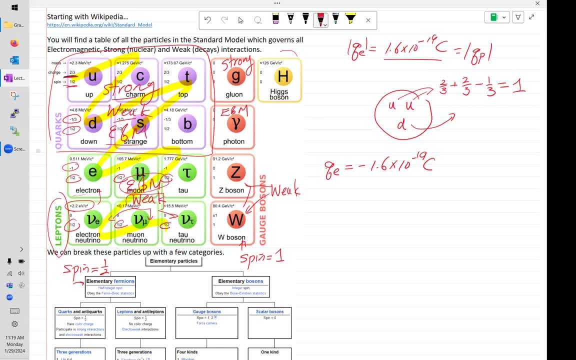 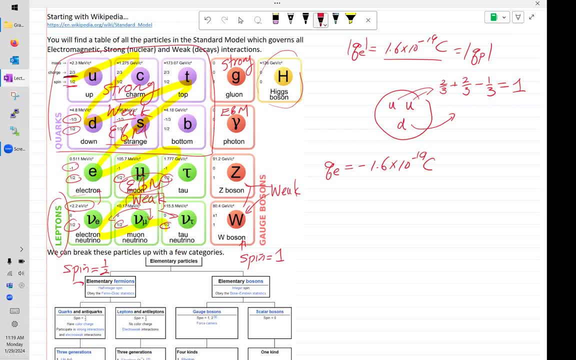 So we're going to further study the Higgs boson, but we haven't confirmed it, But since July 4th 2012,. now we know there's also this Higgs boson right, which is actually a very special boson that has a spin of zero. 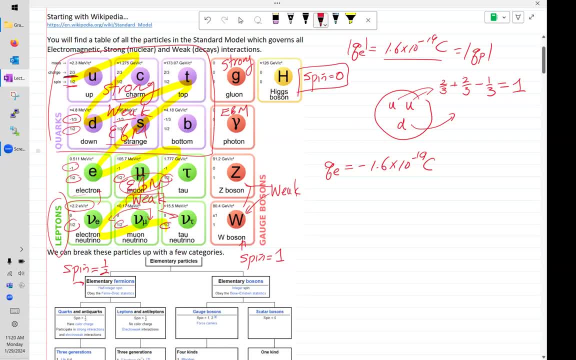 It's the only fundamental particle that has no spin, And we're going to see why that's going to be important when we get to get a little deeper into some of the mathematics. Okay, All right, Any questions about this? I think there's a bunch of lists A. 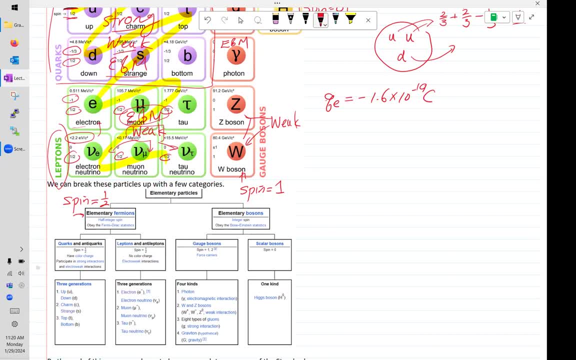 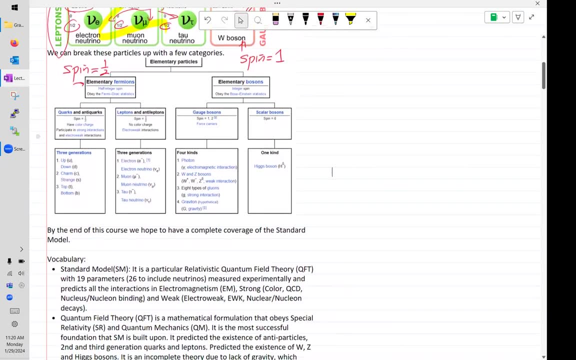 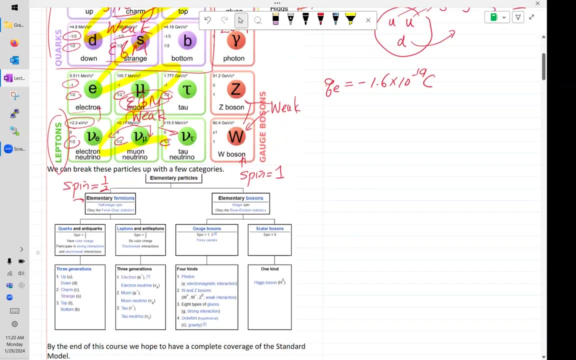 down here. that's on the lecture note, but it's not. I think I talked about most of them already verbally also. Okay, So by the end of this course we're hoping that you're going to understand the interactions between all of these different fermions and bosons and how. that's also 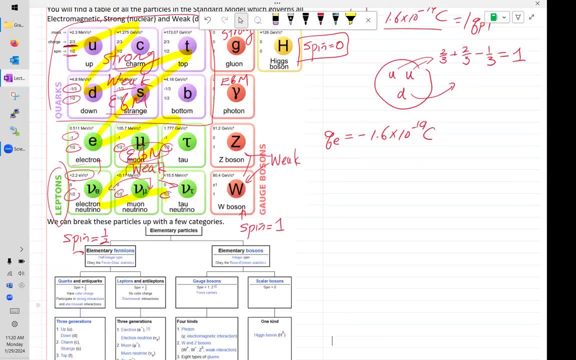 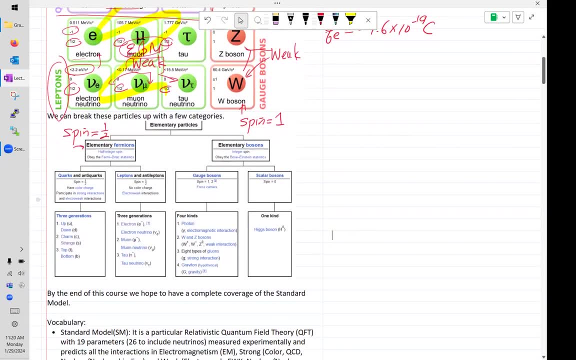 connected to the Higgs boson, which allows particles to gain mass. And this is something that's the goal of this class: to get to the Higgs boson, so that we actually understand why the universe is the way it is right now and why proton have mass, electron have mass and why they don't. 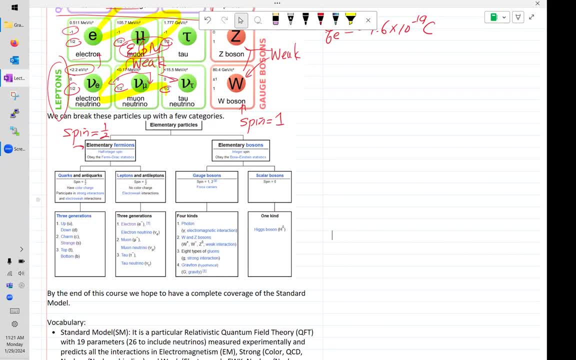 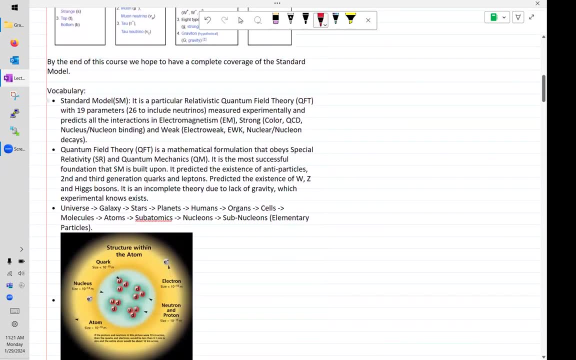 just smash into each other, annihilate and then nothing exists. Okay, All right. Okay, So some of those vocabularies, right, So we have the standard model. So those 17 particles up top are the mass. We have the standard makeup of the standard model, And that standard model is really not a model. 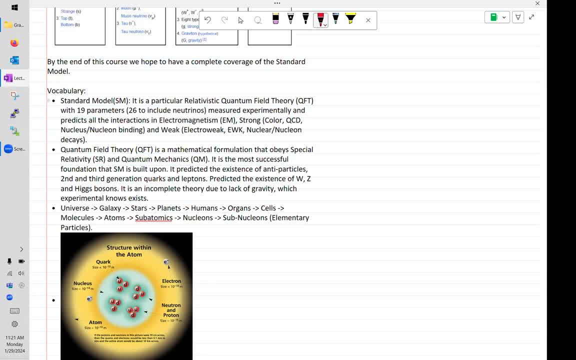 because when you someone say model, you know, oh, you model this, you know- cloud as a sphere or something like that, You're making approximation to things right. In that sense, it is true that we're not. this is not. the standard model does require what's known as. 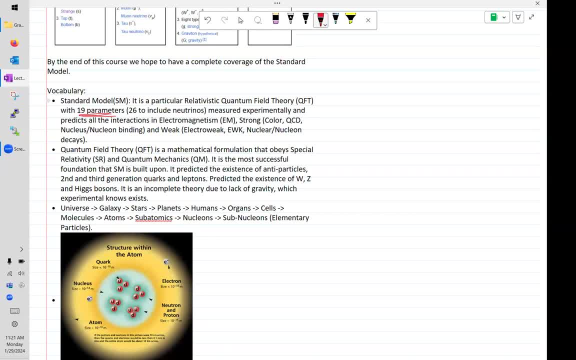 parameters meaning stuff that we measure in experiments in order to figure out how everything works. So it's not like I can just write down a piece of paper and then never do experiment and be able to predict everything about the universe. Okay, So these are experimentally measured. 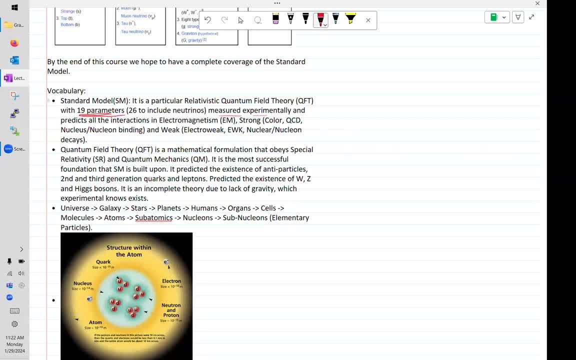 parameters. So there's 19 of them And most of them are like the masses- Okay. If you include the neutrino, there's actually 26, also Okay. And all of this governs the electro electricity, magnetism, the strong interactions. 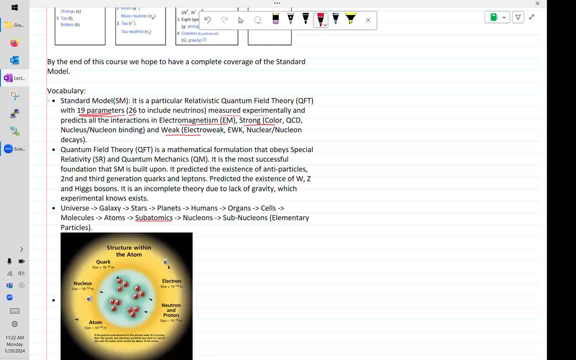 And then the weak interactions. Okay So- and all of this is great- based on this um theory, or or um call quantum field theory, which we will not do in this class, cuz that requires so much more math than that We can, we'll, we'll just be here, you know, all semester, just to get to the 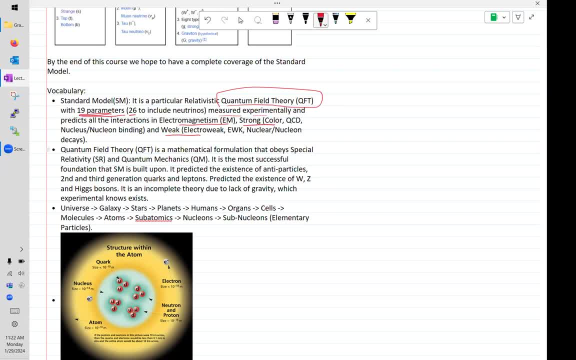 beginning of the standard model. Okay, Okay, But we'll we'll. the way we're gonna try to formulate things is that we're gonna take the stuff that people are already learning from quantum field theory and we're gonna apply them in the way that it obeys special. 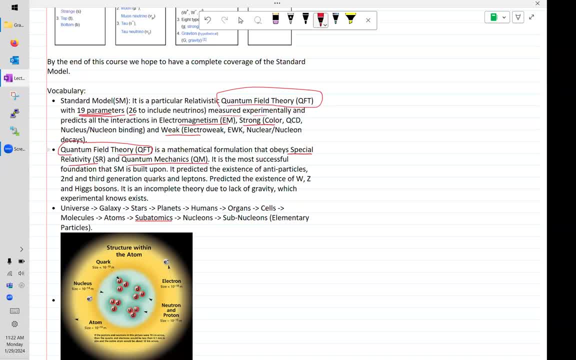 relativity and quantum mechanics. Okay, We're gonna combine special relativity and quantum mechanics together. Okay, And remember, special relativity is kind of like the first part of modern physics, right, Where you do time dilation and length, contraction and all that stuff. Okay, 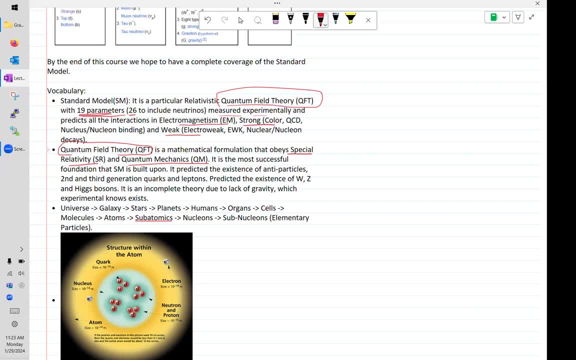 Quantum mechanics is sort of like the end of modern physics, where you're doing, you know, um once again the angle momentum of a hydrogen atom or quantum tunneling and all that, all these um unintuitive processes that happen in real life, that that quantum mechanics predicts and 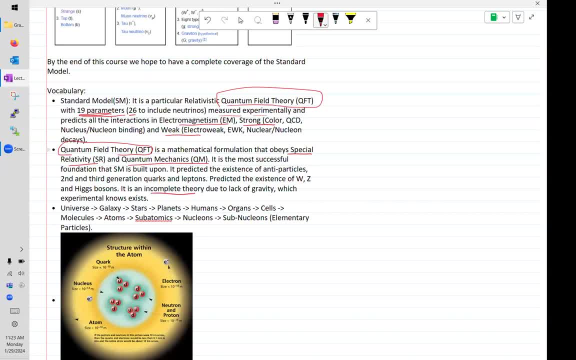 we're actually able to measure. Okay, As I mentioned, this is still an incomplete theory because it does not have gravity in it. Okay, So gravity is important, right, Cuz that's the only reason where I'm standing here and not floating in space. 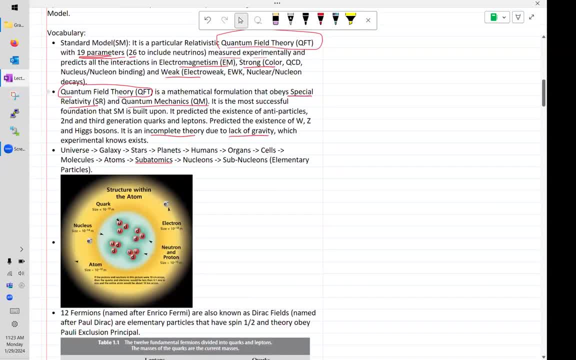 Okay, But just to think about the scale of the standard model, Okay, So okay, The standard model has prediction that tells you about the entire universe. It tells you how galaxies form, It tells you how stars form, How planets form- right, And you know how human beings behave, you know how we work, basically. 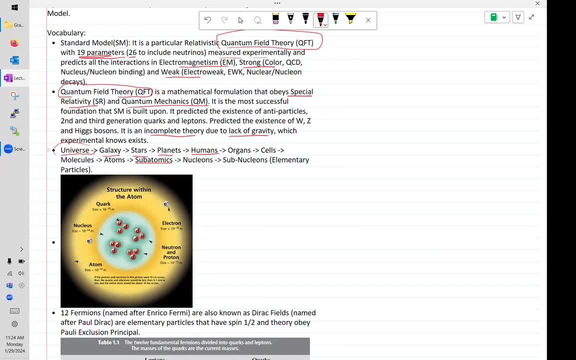 you know all the electricity, magnetism inside us, right, And it goes all the way down to the atomic level, sub atomic level, meaning inside an atom, right? How does you know? basically, the hydrogen model, uh, hydrogen, uh, add. a model is: 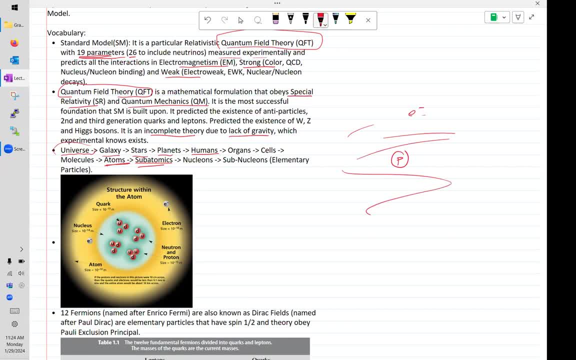 electron and a proton and the heart. and the electron is kind of a little fuzzy cloud around. right, that's already subatomic, because you're looking inside an atom and how that works, right, okay, but also nucleons. nucleons meaning protons and neutrons. you can write those out, i can with. 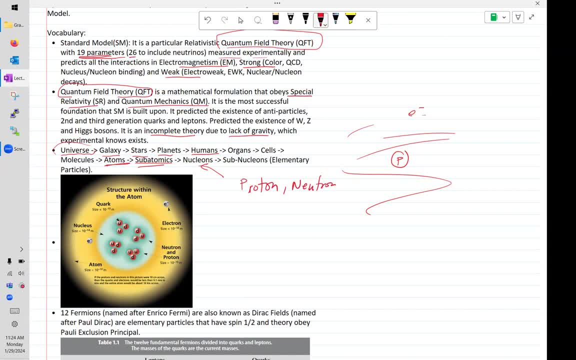 the 10 neutrons. okay, there are others, you know nucleons also, but not even that. right inside the proton, right, as i mentioned, inside the proton there are up quarks and down quarks and there are gluons and we're going to see why these. these are a little squiggly line like this: 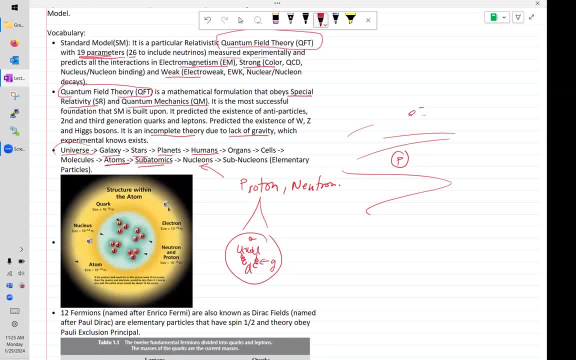 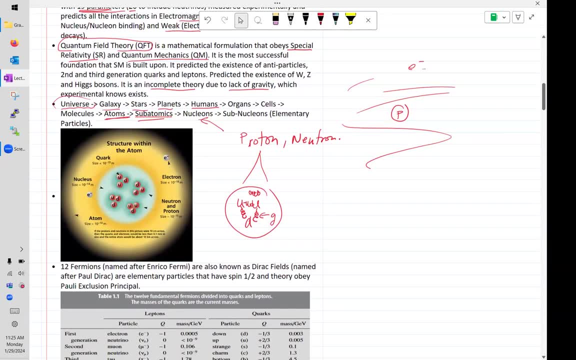 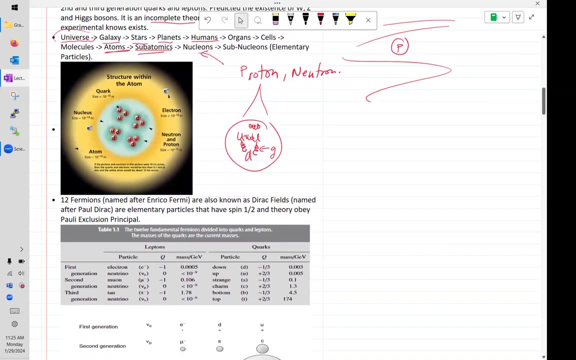 linking them together. okay, there's actually a lot of them inside, inside a proton, okay. okay, and that's how, that's the range that the standard model can actually make predictions on, and which is, you know, a already a fantastic thing. and if we get gravity into it, 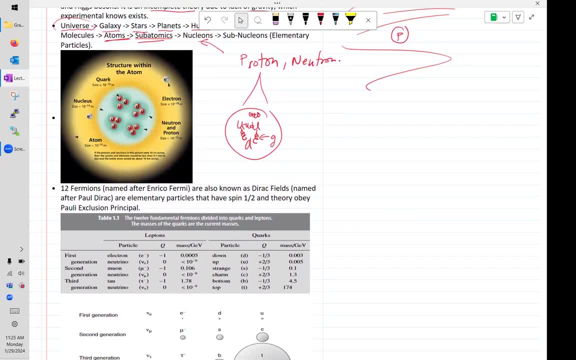 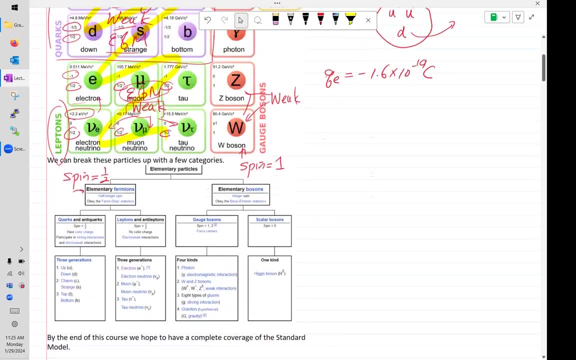 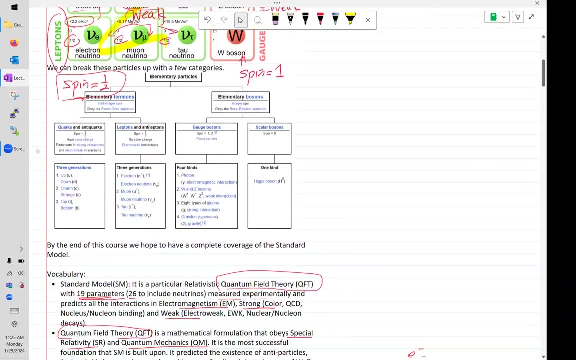 then then, then we're done. it's like finish our homework, okay? um, as i mentioned, there are uh, 12 fermions. so remember, up here right, all the stuff on the left right, the all the quarks, all the leptons, they're considered fermion and they're special because they are. they all have spin one. 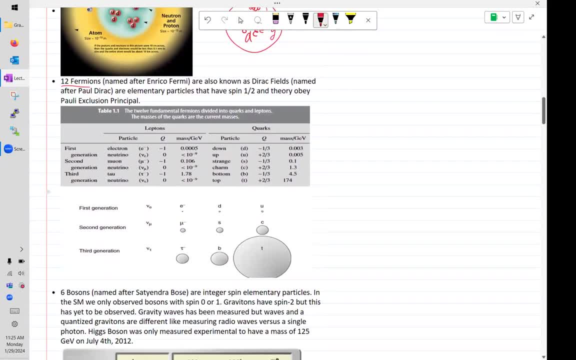 half. okay, and here's the list in the textbook of all the fermions. we're not going to go through all of them, so you should read that yourself. but this, this picture is kind of neat. uh, we're where it's, showing you, kind of like to scale, how big, how massive right the top quark is to this t. 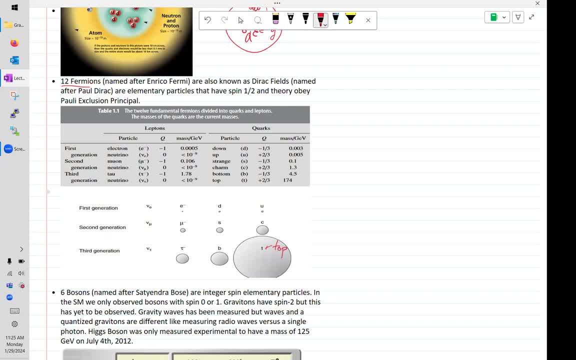 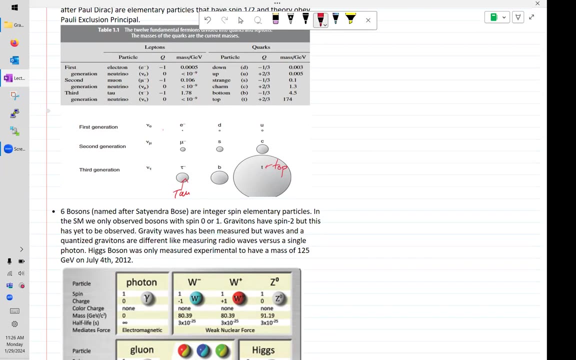 here and it stands for the top quark, okay. and then the tau is down here. this is a lepton, okay, this is the tau lepton, okay. uh, the different scales and how, how, how, how, how massive or less massive things are to each other. you notice that the stuff on the left here, right, all the neutrinos. 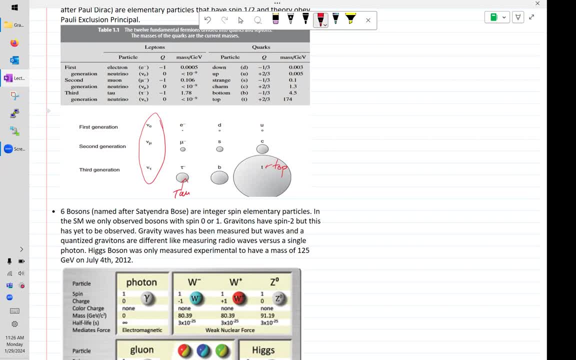 are basically massless, right, okay, and we have the first generation right, which has low mass. as you increase in generation, you get more and more massive. okay, hopefully that pattern makes sense, okay, okay, right, the uh, the neutrinos are kind of special because we haven't measured their mass, so we 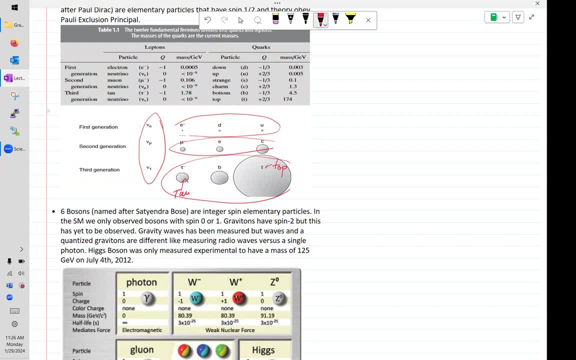 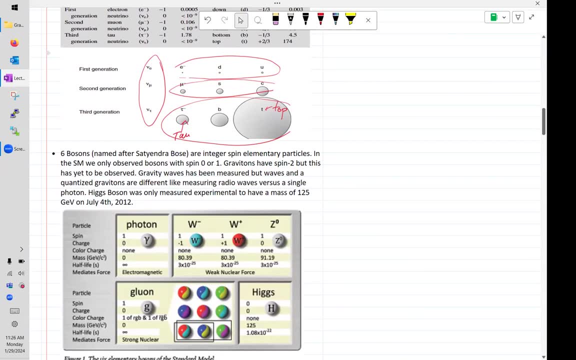 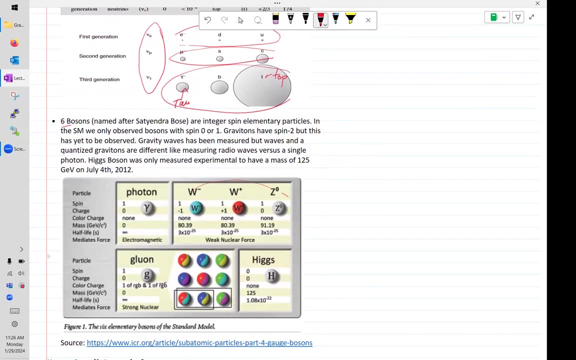 we're not, you know, we're not sure how to actually arrange them, okay, um, this is actually a a fundamental problem in neutrino physics, that we're still doing experiments to try to learn. okay, and, as i mentioned, there are the six bosons. so the bosons are, you know, the photons, the, the w and 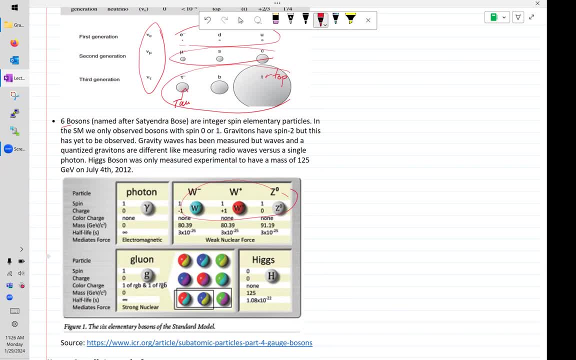 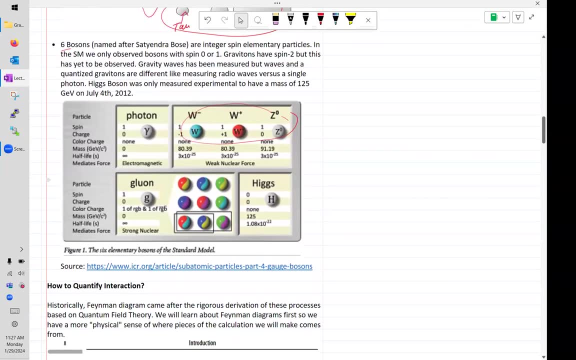 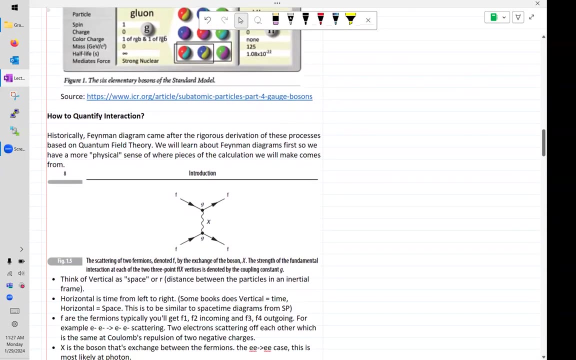 the z bosons and then the gluons, which has these like kind of cool billiard ball type of multi-color thing, and and we'll see why it's actually very important for them to have two colors. okay, otherwise none of this actually works. okay, okay, but the goal of this uh lecture is to figure out. 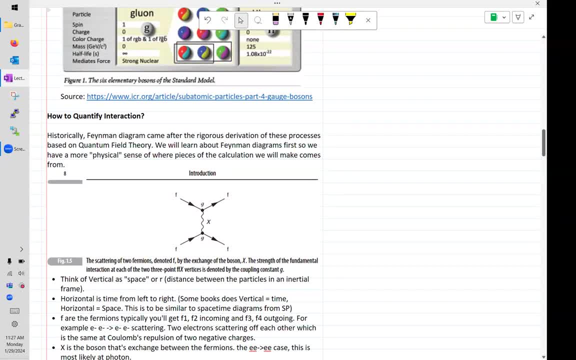 how can we at least qualitatively quantify, well, qualitatively figure out what their interaction is, what is allowed, what's not allowed, and and then we're going to kind of get into the quantification of it. okay, so historically, um, uh, these things called Feynman diagram, which is this diagram down here. okay, um came after a lot. 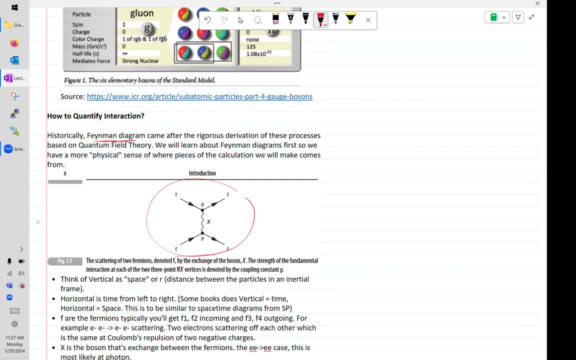 of really rigorous uh process, uh work that's done by theorists and in quantum field theory, in order for us to, in order for for for us to have these Feynman diagram for to get a more physical sense of where you know how strong you know each of these. these um interactions are strong as in, not the strong. 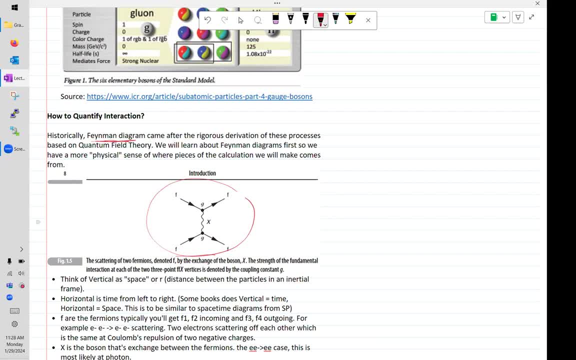 force strong, like how, how often they happen, how problem, how probable it is right, and which one is allowed, which one is not allowed. there's certain things that are not eight, that that are not allowed, okay, and and so this little diagram, you know, basically, is a way for, especially for. 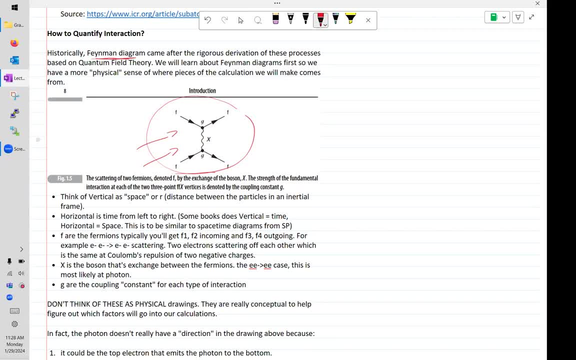 experimentalists like myself to understand what actually was happening when, um when, there are interactions between elementary particles. okay, okay, so I'm going to erase this because I'm actually you need to write on this. okay, so think about the vertical space. um, it's in this book, at: 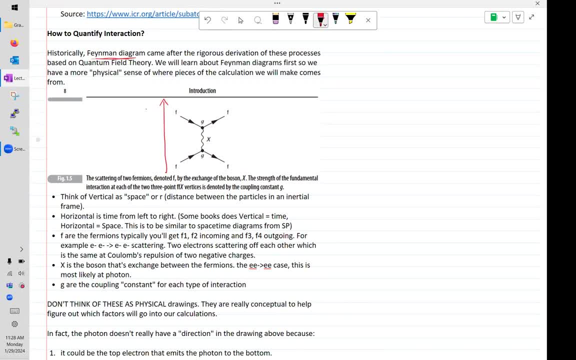 least as kind of like um, the vertical axis, as like space, basically like a distance between the two particles, okay, and then the horizontal is time, okay, okay. so think about this as like distance between things, okay, and- and this is a very qualitative thing- this, this is actually not how particles actually 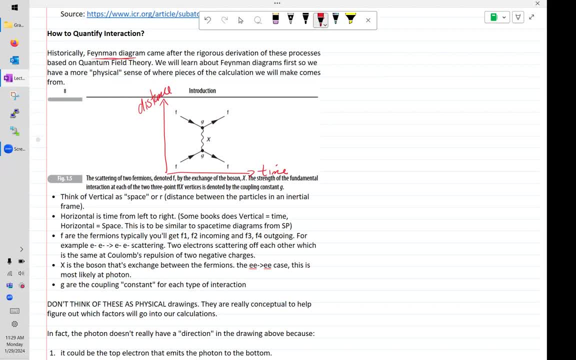 interact with each other. they don't come in at exactly at this angle until we hit each other, right, okay, okay. so the vertical as kind of like distance between things, and then horizontal is time. um, some books do make things the other way, so that's just to uh, mess with you guys, so we'll. 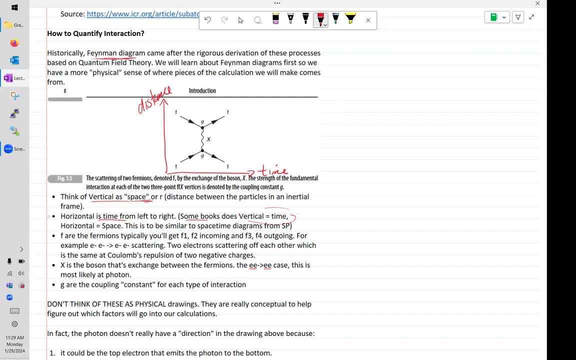 have some of the textbook will have time on the vertical and then distance on horizontal, uh, and that's to to agree with like space-time diagrams and stuff like that. so me, so maybe there's more theoretical textbook, we'll do it the other way, so don't don't be surprised, okay. 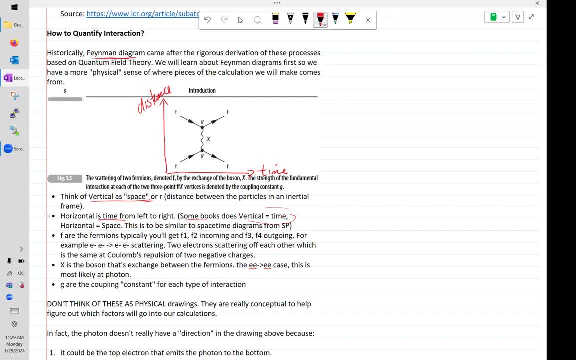 so let's figure out which convention they're using and use that one for that particular book, okay, okay. so these F's here, right, they stand for the fermions, okay, okay, and and what's happening here is that a fermion is coming in, another fermion is coming in, so let's call this F1, F2. 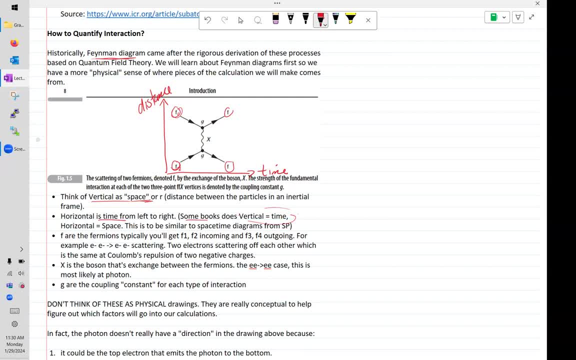 or something like that. right, and what's happening is that they're scattering each off each other by exchanging a some sort of boson. okay, so these are the fermions, so these are the bosons, uh bows. okay, I'm gonna write these out so you guys have the. 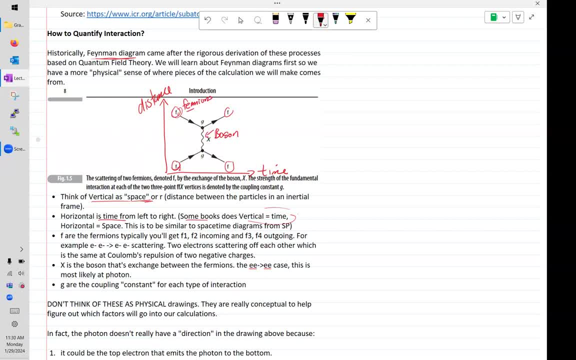 okay, okay, and this is how all interactions happen, which is sort of neat. um, there are uh bosons that couples to each other and- and this is going to turn into a big mess when we get to QCD, but at least at the um, with the first type of interactions we're dealing with, which is going to be the quantum, 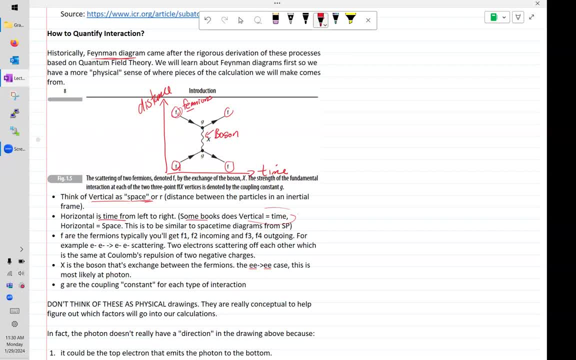 dynamic, meaning we're only going to deal with electricity, magnetism. um, these are going to be the type of interactions that where you have fermions and they're going to exchange some sort of boson to scatter, to basically bounce off each other. that's the the reason that that happens because just imagine if you, you and your friend- is walking on like a ice rink or something like that, and one of you throw a bowling ball in another right, they're going to be bouncing off each other, right, just to conserve the momentum. so that's why they scatter off each other like this. 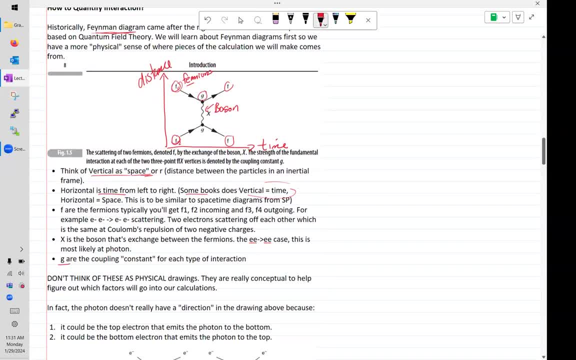 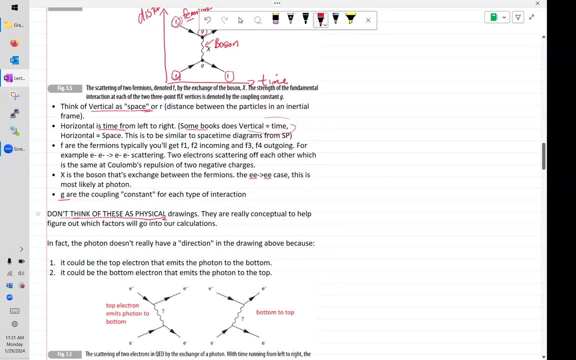 okay, this little g here stands for the coupling constant and for each type of interaction, meaning electricity, um, electricity, magnetism. the strong, the weak, they would have different coupling constants between them, and that basically scales how often and how probable these interactions are okay, and so one thing that the book also warns you is that don't think of these as physical. 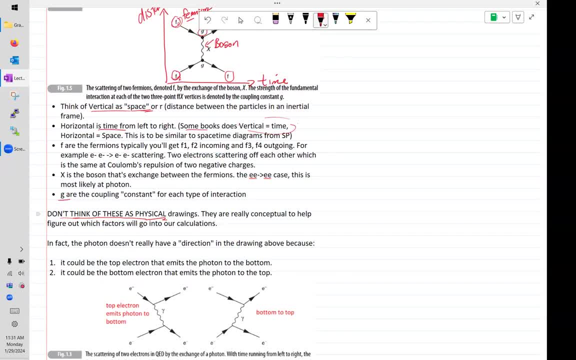 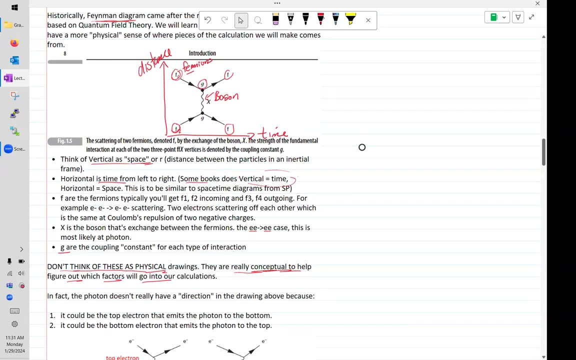 drawing. they're very conceptual. okay, it's just so that we're using these, these diagrams, in order for us to conceptually figure out what factors goes into our calculation. okay, right, what is the momentum coming in here for these fermions? what is the um, the coupling between them? okay, which boson is being exchanged between them? okay, 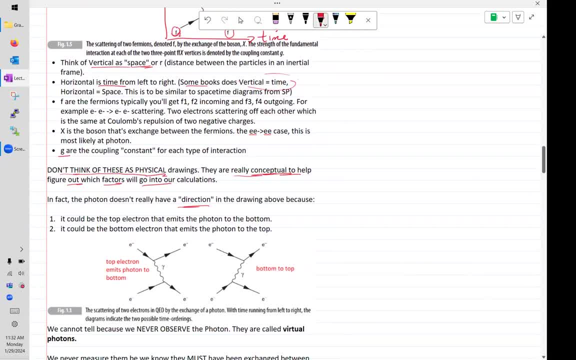 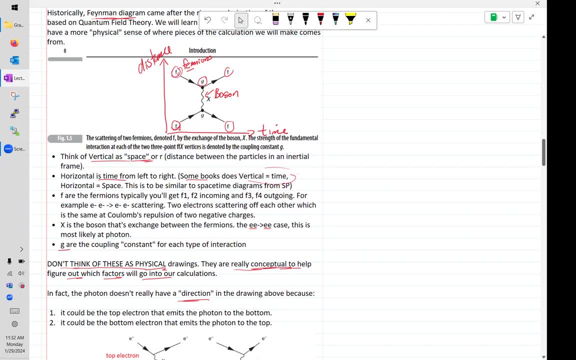 in fact, these diagrams don't really have a direction in them. okay, you can see on top of this diagram this gauge boson between them, right, this one, let's highlight that right. right, it's drawn vertically, right. okay, so if you have a time axis, that's going. 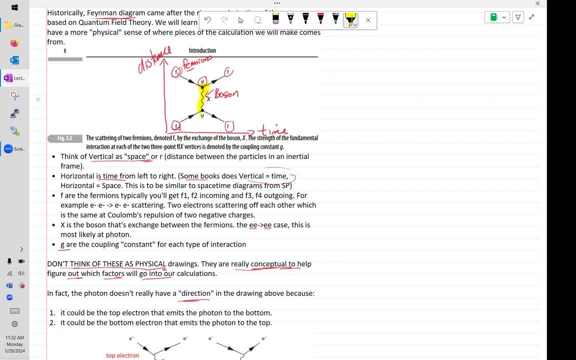 horizontal. if you draw a vertical line, that does anyone know how fast you should you need to be going in order to do that. if you're able to traverse some space in no time, what is your velocity? people are shy because it doesn't make sense, but that's okay. that's it, i'm sorry, go. 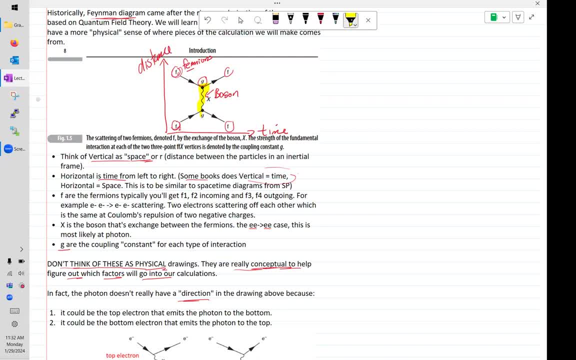 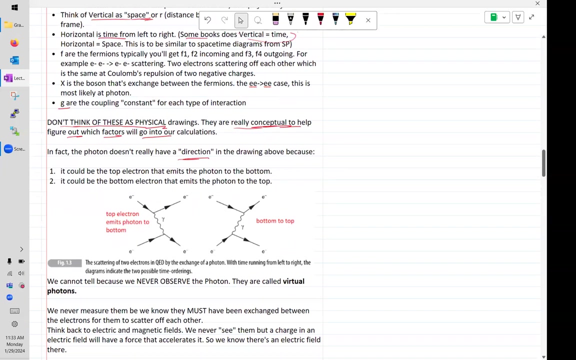 ahead the speed of light. even more than that. it's actually infinite, right? right, when delta x is, you know, non-zero, and then delta t is zero, right, because the horizontal axis is time. right, it's one. some some number over infinity is always going to be infinity, okay, so that makes no sense, right? okay? in fact, what really happened is that, let's say you. 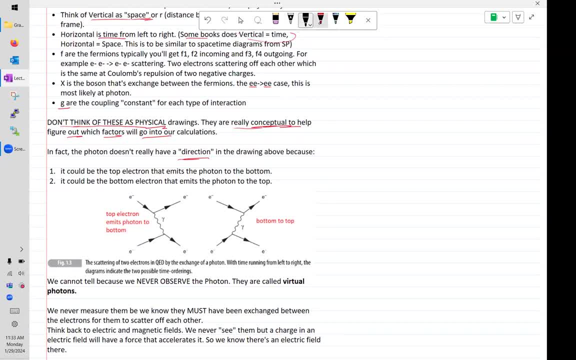 have two, two electrons scattering off each other like this. down on this, the second diagram, the photon is emitted from maybe electron number one. i'm going to label them one and two, so it's just i can talk about them right- being emitted from electron number one and got captured by electron number two and therefore the two you know are exchanging. 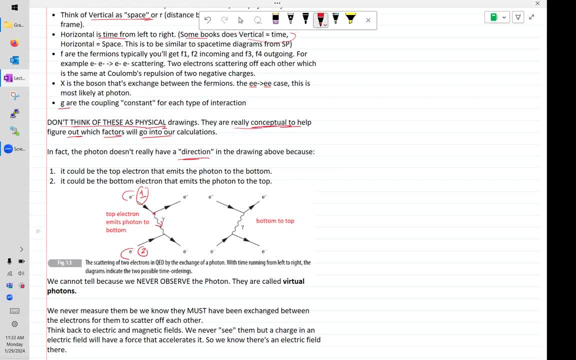 the bowling ball they're throwing between them, right? okay, so you have some initial state with some electron coming in, right, two electrons coming in, two electrons coming out. okay, you never really observed the full the photon between them, right, because you don't. if you've observed the photon between them, you actually interrupted that interaction, the 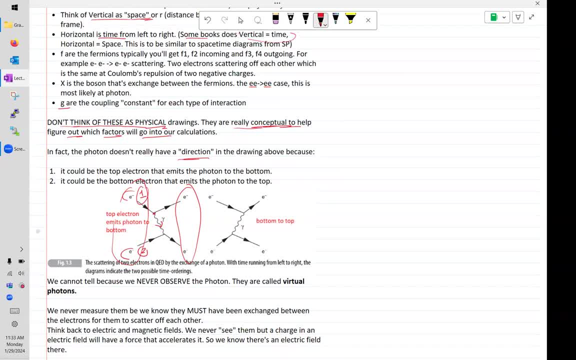 bowling ball got captured between the two, right? what could have happened is that, well, maybe electron number two is the one that emitted the photon right and shot it out to electron number one, so this could have been in a different order, right, but what happened is that in experiments or 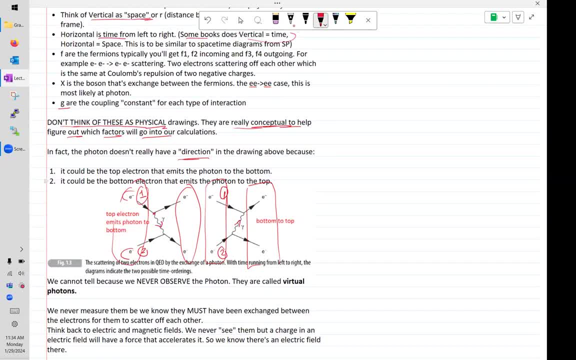 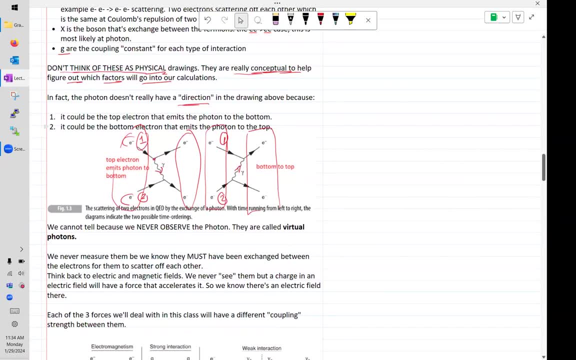 in real life, right, what was going to happen is that you just see two electrons bouncing off each other. you never actually see the photon between them, right, okay, when you never observe the photon, these are called virtual photons. in fact, in general, virtual particles are going to be a part of inside. 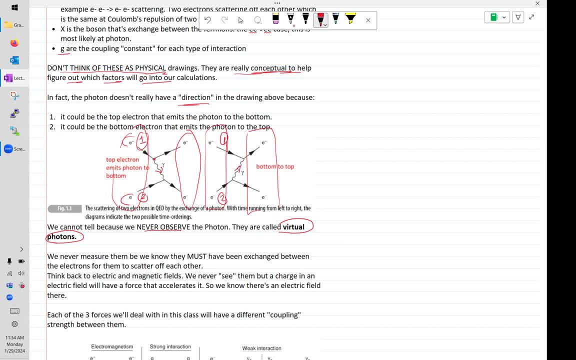 these, uh, Feynman diagrams, so that you never actually observe them, but you know that they have to been. have been there in order for the two bowling to for the electrons to bounce off each other, right, okay, if you have two ice skaters skating parallel to each other, right? all of a sudden, the two just. 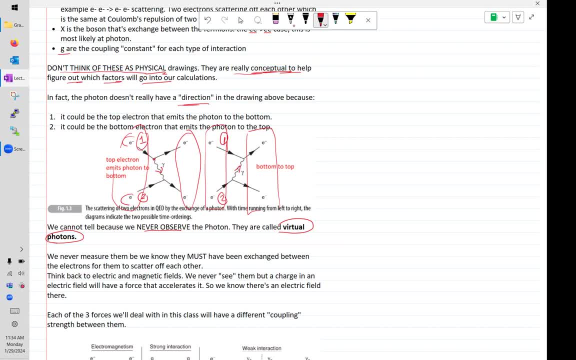 start veering off from each other. you know that they threw some bowling ball between them, right? I keep using this bowling ball analogy. I don't know if that works. throw a rock between them, something, or bag, okay, okay, okay. so that's the idea that these virtual particles are. 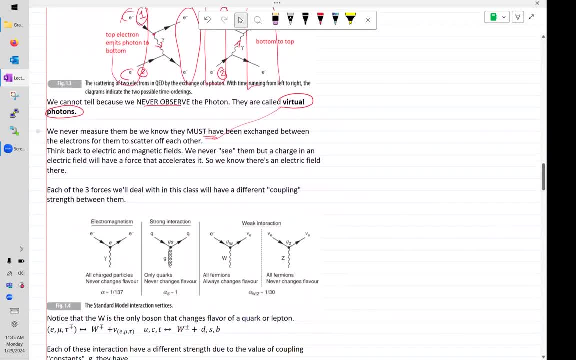 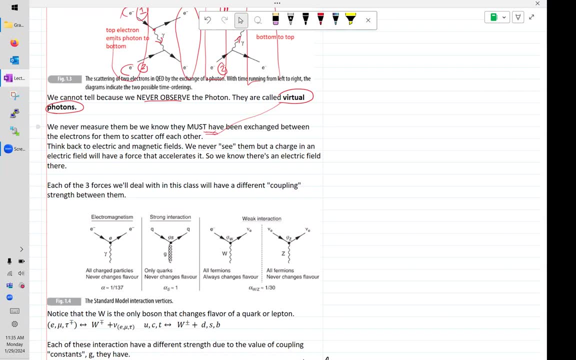 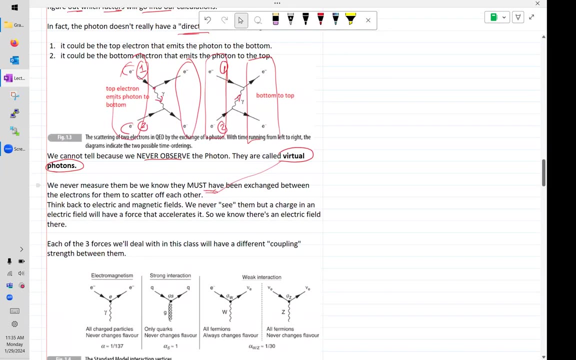 never observed, but we know they have to exist, okay, okay, so, and this makes things conceptually a little bit um, maybe misleading, I don't. I don't, but the way we draw the Feynman diagram is that we always make this photon vertical. okay, it doesn't mean it is traveling. 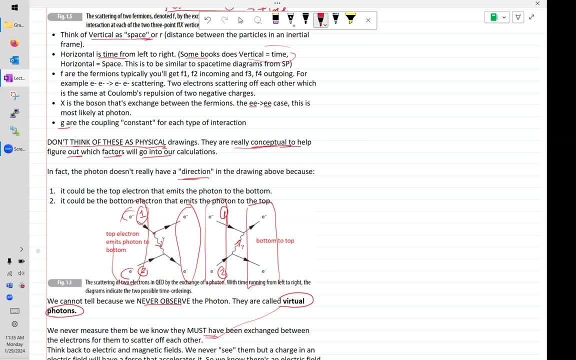 at Infinite's velocity. it's just that we can't tell which one is the: the electron one emit the photon or the electron to emit the photon. we don't know what time order it is okay, so we just take the average, we just make them vertical, so we don't have to think about it. 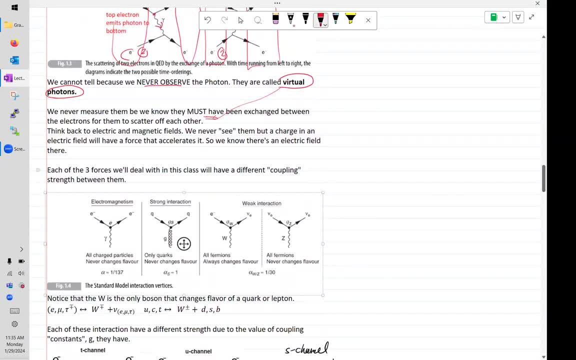 like that. okay, in fact, okay for the three fundamental forces we're going to be dealing with. okay, there are going to be these Feynman diagrams will be made up of these vertices. okay, these are different vertices, so you can see that this one up here downside this one down here is. 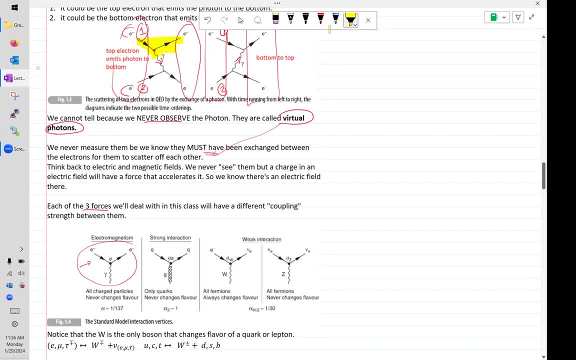 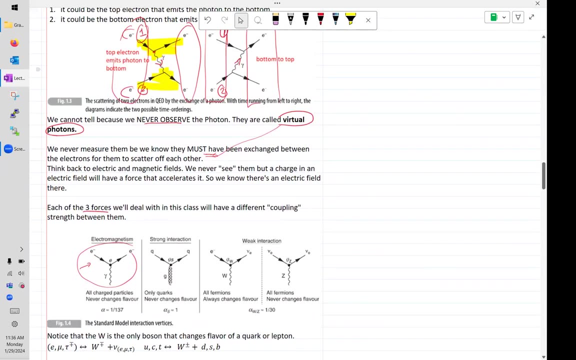 actually the top half of this interaction, okay, in fact it's also the bottom half, right, but upside down, right, okay, okay, so that's the electromagnetic interaction vertices. so if you put two of these together, you have an electron, two electrons scattering off each other, right, okay? so some of the rules that we use. 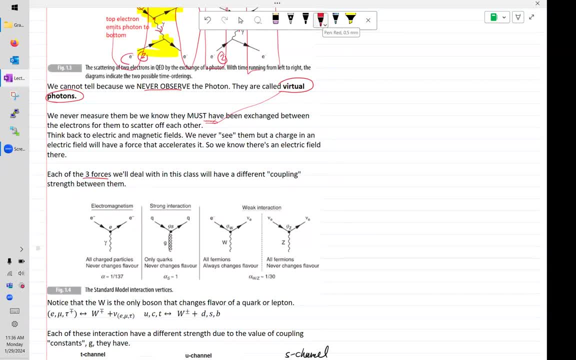 to make sure that people are clear, what's what's being shown on this diagram. is that right? you have your particle, that's coming in, okay? an electron is a particle, not an anti-particle, and we're going to try to figure out how to deal with anti-particle in a second here. okay, okay, since. 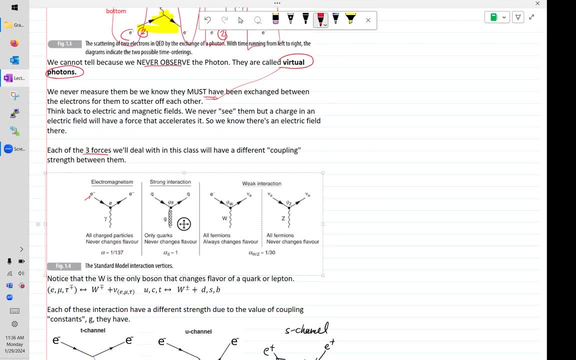 electrons only interacts electromagnetically and weakly, so we don't have to deal with a strong version of this. okay for the electromagnetic interaction. it always gonna, it's always going to emit a photon. okay, and then, since they emitted a photon, right, if, if this electron was to keep? 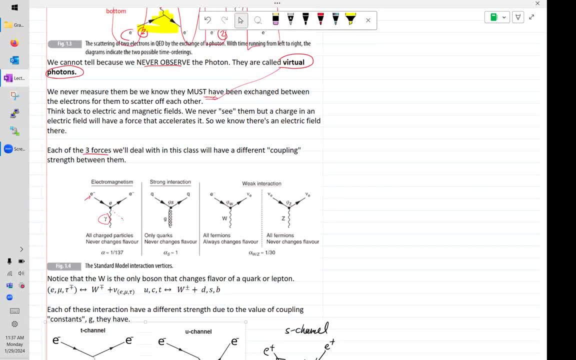 going without emitting photon, it just go in a straight line. that's sort of how you want to think about it. okay, but it did emit that photon. so in order to conserve a momentum is kind of: have this little you know pink in, Okay, Okay, But you know it still remains in electrons, It's just, you know, shot off, you know a little bit of momentum or energy, however you want to do it, Okay. Okay, Let's not talk about this stuff yet And I will talk about that in a second Okay. 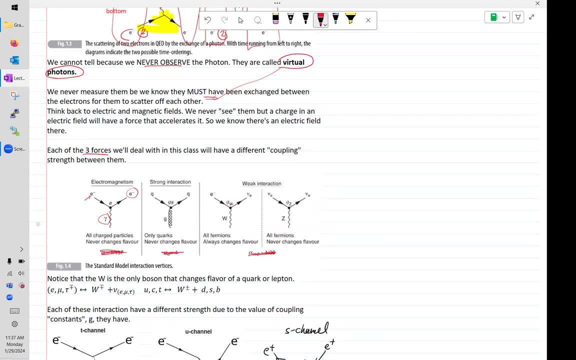 So for the strong interaction, okay. similarly, anything, all the quarks, okay. that's why these are labeled Qs instead of F. Okay, Instead of shooting off a photon, it'll shoot off what's known as the gluon. Okay, Remember, the gluon is the boson that couples to the strong force. 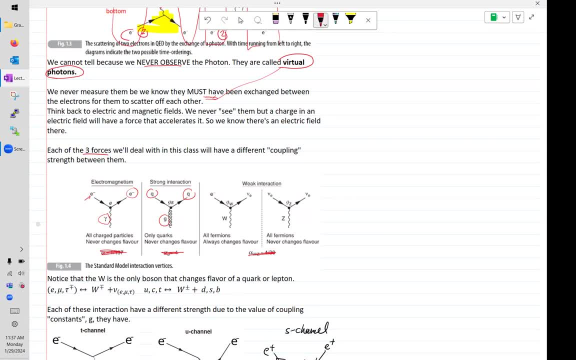 Quarks is also charged, right, You know. down quark is negative one-third charge, Up quark is positive two-third charge. So quark can also be charged. Interacting with electromagnetic also right, So I can. why is this doing that? Okay, So you can also draw maybe a up quark scattering off, having a vertex like this also. This is also possible, Okay, Okay, Because this has some electric charge. 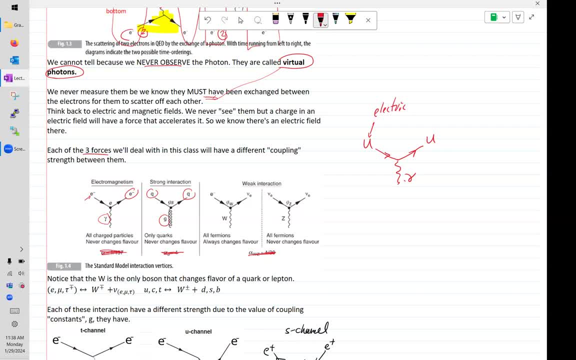 Anything that has an electric charge can emit a photon. Okay, Okay, Sorry for the bad writing. Try to be quick. Okay, The weak interaction actually has two types. Okay, There's the one that involves the W. Okay, It looks very similar. And there's the one that involves the Z boson- Okay, 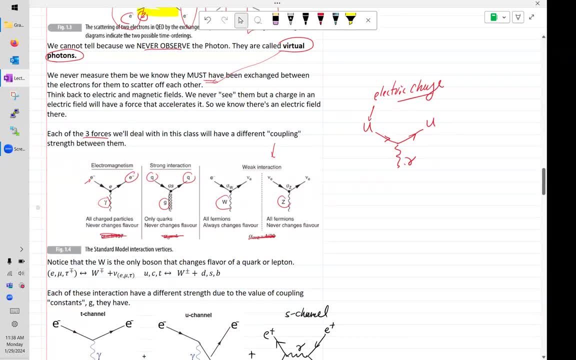 The W boson is special, It's because anything that any vertices that involves the W is always going to change the flavor of the particle. And what the hell is a flavor? Okay, Is it like strawberry orange? you know banana. 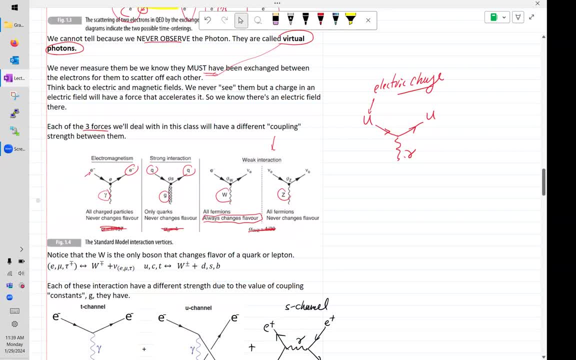 Right. By flavor we mean, you know, is it an electron, Is it a neutrino, Is it an up quark and a down quark? Right, These are different flavors And technically like, if you're comparing, like the muon to an electron, that's also kind of a flavor. But it's better to refer to them as different generation of the same flavor. Okay, Okay. 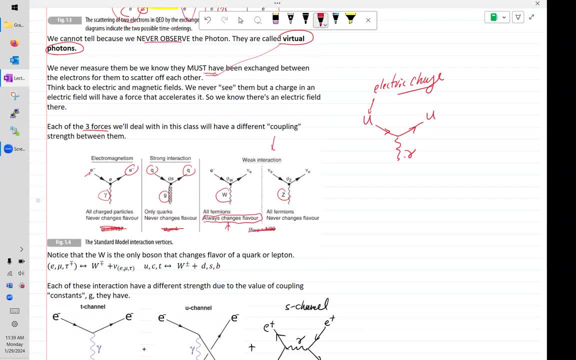 So the reason for that is always- It always changes flavors. So look at this little diagram here. Right? So a W boson has an electric charge or either plus or minus one electric charge, Okay. So if it emitted that plus or minus one electric charge, in this case it's going to be minus. Okay, Let's just put a minus here. 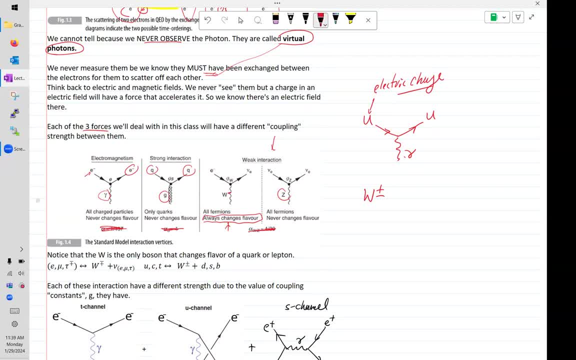 Okay, Right, That electric charge cannot remain afterward, Right. You already gave up your one charge, so you cannot have a charge afterward, Right? That's why it comes out as a neutrino. In fact, this one is going to be a electric neutrino for the time being. 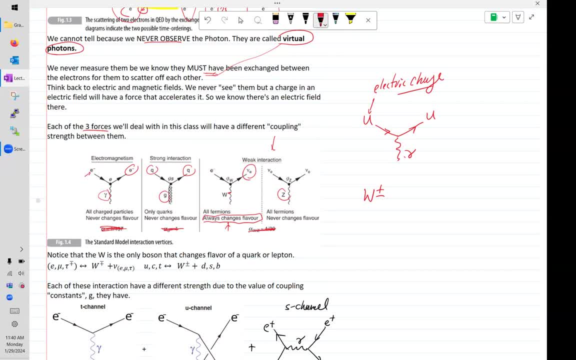 And okay, Okay, That's how you change charge leptons into neutral leptons, All right. Electrons to neutrinos: Okay. Same thing with muons, Same thing with taus. Right, They would each create their own generations of. 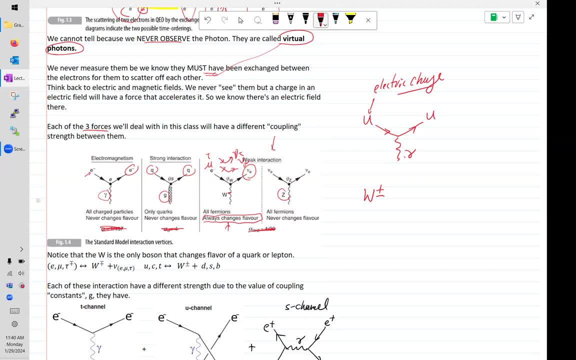 of particles when they emit electrons. they basically convert one particle to another, one flavor to another. Okay, The Z boson does not do that. Okay, This is one of the things that technically in the rulebook you could have done it, but we never observe it to happen. Okay, 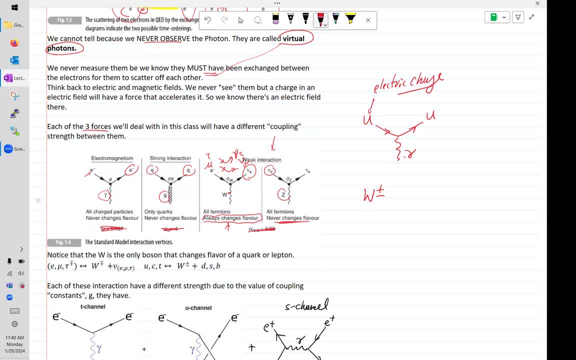 All right. So in this case it's basically a neutrino emitting a Z boson and then going off as a neutrino also. It doesn't change to some degree. Yeah, a z boson and then going off as a neutrino also. 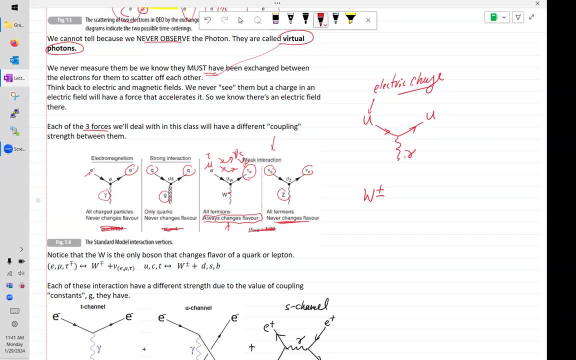 It doesn't change to some degree. Okay, something else, okay, okay. so, um, just, i want to give you guys an example of the strong version of this, the quark version of this. so so, if i have an up quark right which has the charge of plus two-third right, i'm actually putting it at the wrong place. i'm just going. 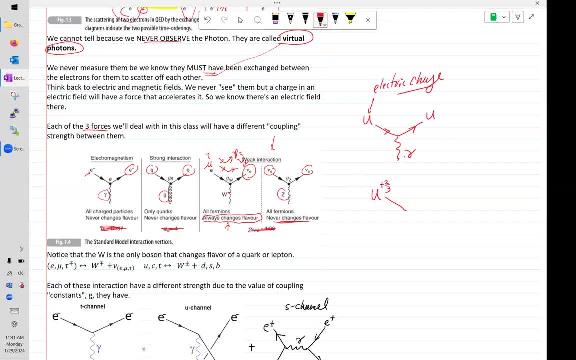 to write it in the right place. then plus two-thirds. okay. if it comes in, emits a w plus right. what has to be the charge of the thing that comes out? anyone on zoom or anywhere? you got two-thirds, you lost a full charge. what has to be the remaining charge here? negative one-third, yeah. 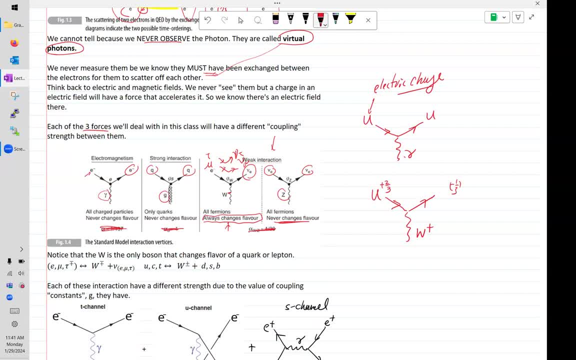 and what type of quark would have a negative one-third, a down quark and also the strange quark and also the bottom quark, okay, and these all are possible, okay, but mostly it's going to change into a down quote. okay, i'm going to see this in when we get to the qcd part, much, much later. okay, all right. 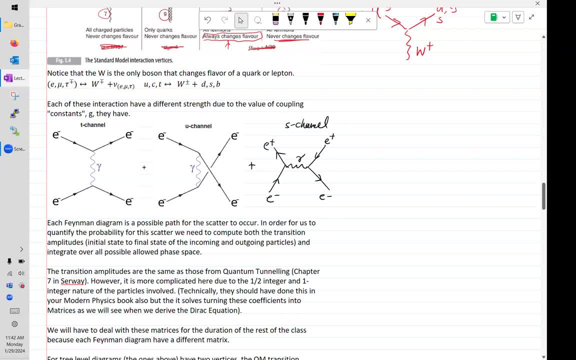 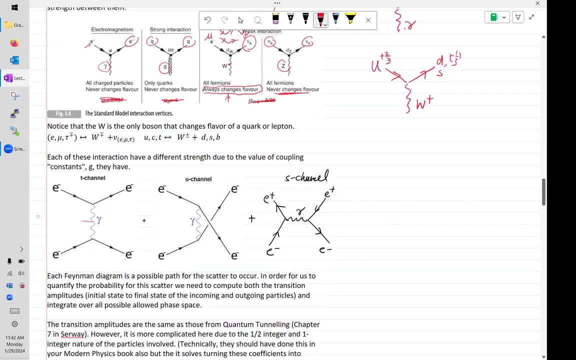 so, um, just to finish up with these interactions, okay, when you combine these two things together, you can imagine combining them in different ways. so this is um. this diagram here is known as the t channel, meaning it's the one we've been looking at a lot of times when we've been looking at a lot of times when we've been looking at a 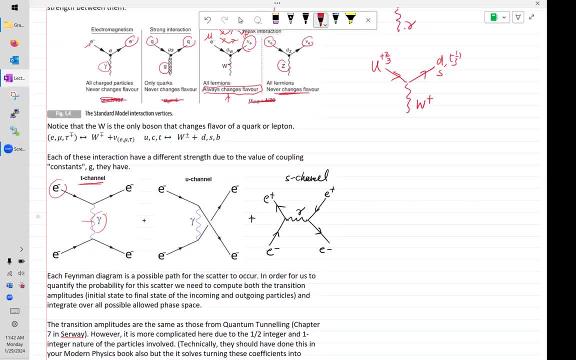 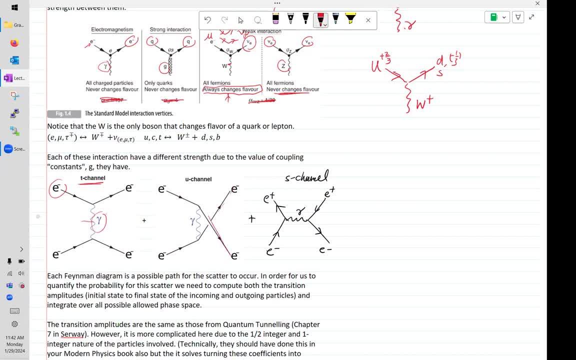 you know, swap the outgoing particles, right. if we call this electron one, electron two, right, this is still electron one, this is electron two, right. but you can have a case where one and two comes in, but then two, sorry, one goes out this way and then two goes out that way, that's. 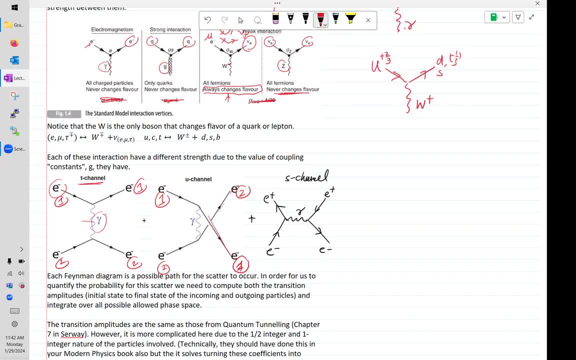 this way and then two goes out that way. that's actually technically a different diagram, okay, okay, and for some reason the book didn't put this here, but this also was known as the s channel, where basically what's happening is that you have a positron, a positively charged electron. 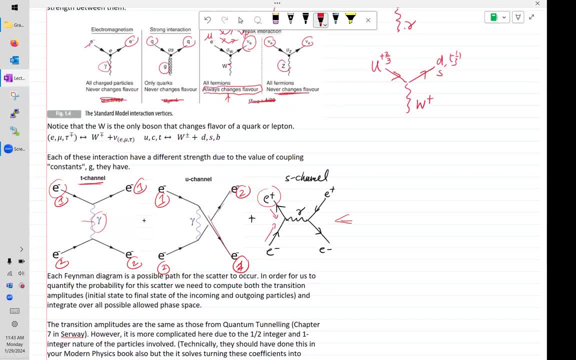 flying in here and then annihilating with a electron, creating a photon and then, and then emitting a positron and an electron afterward. okay, okay, and this brings up sort of a you know interesting case. you notice that even though the red arrow here oops, it's not on the board yet. 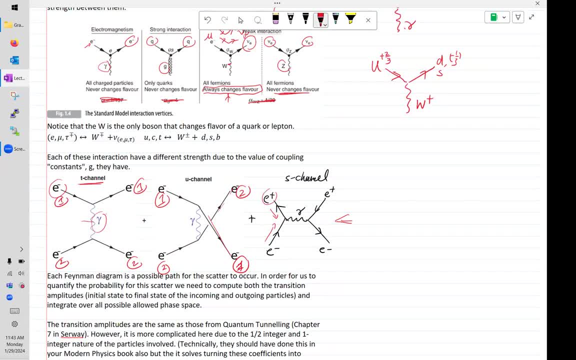 some reason. okay, the positron here. right, i say it's coming into the vertex. right, i'm drawing the arrow going out. okay, anytime there's going to be an anti-particle, okay, it's always drawn with the arrow going out, so that way you can just have so. so these arrow are actually tracking like particle-ness. 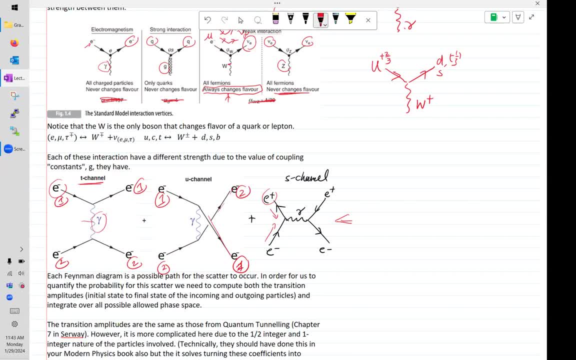 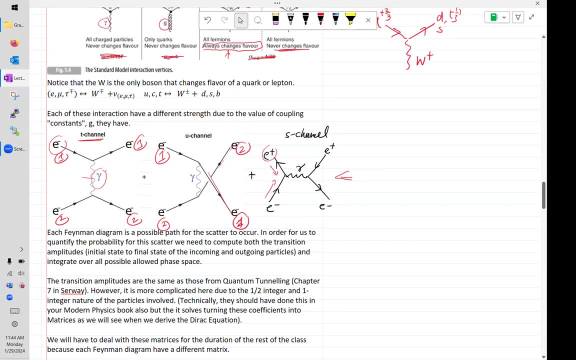 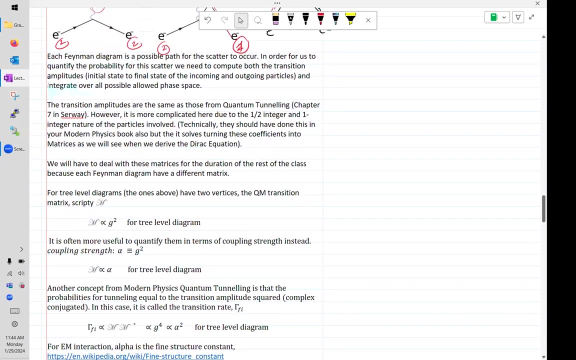 moving around. does that make sense? and we're gonna. we're gonna see how, why, why, why it is completely necessary for us to have anti-particles in our universe and um, and that's the only way these will work. okay, i guess i don't have time to do the little exercise today. so, alex, i don't think we're. 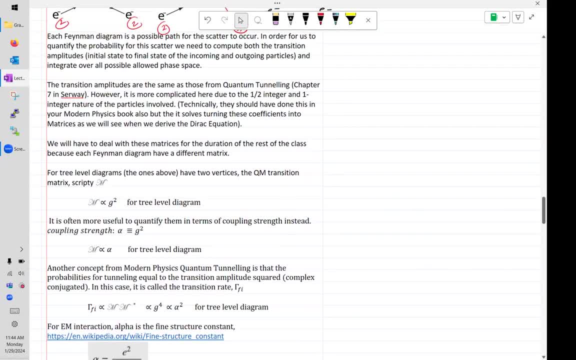 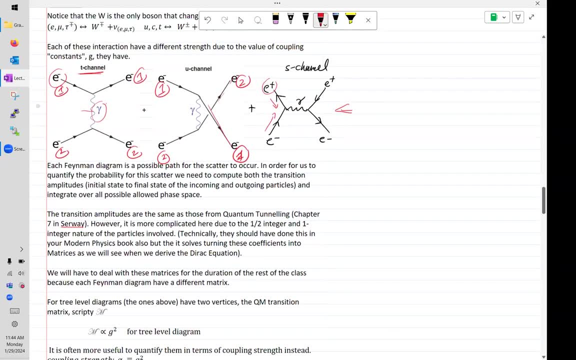 gonna be able to do the little um exercise today, but that's fine, we'll do that the first thing on wednesday, okay? um, so each of these diagrams are going to be moving around, and they're going to be moving around, and they're going to be moving around, and they're going to be moving around, okay. 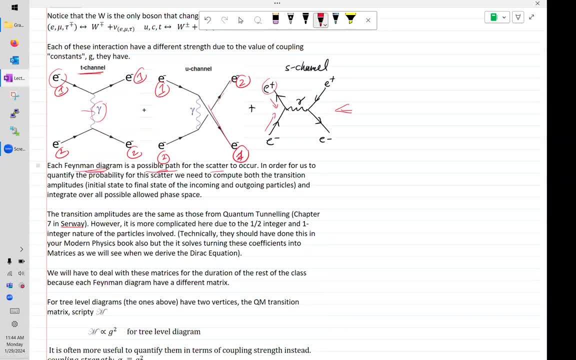 feynman diagrams are a passable path for these scattering to happen, right. so if you, if you have electrons, two electrons, okay, both of these are possible ways for the scattering to happen. okay, but what happens is that when you measure them outside, you don't know which one is which. 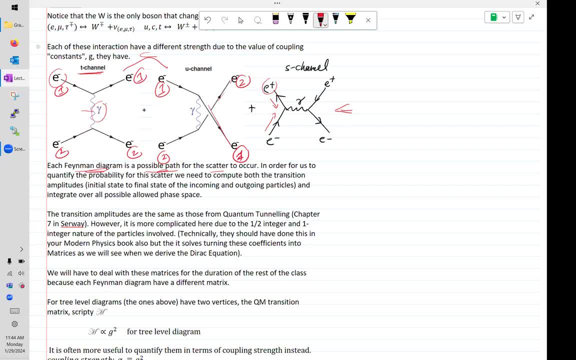 right. you don't know if- especially since, if they're identical particles, right, one electron looks exactly like another electron. so when these comes out, oh well, in the experiment, you don't know whether or not it's the t channel that the scattering happened off of, or the? u. 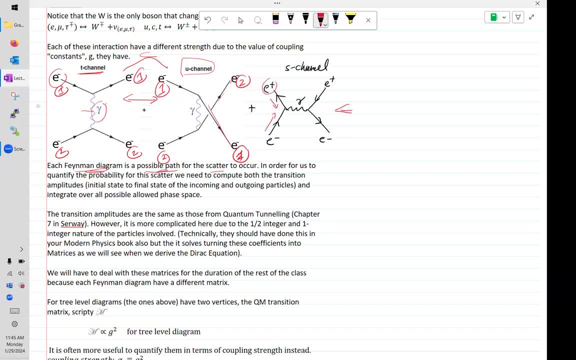 channel. okay, in quantum mechanics, when you don't know which one is which, what do you do? because i remember you add them? at what between them? does everyone remember those keywords? anyone on zoom you when you, when two processes happens right at what? sorry, can you speak loud? 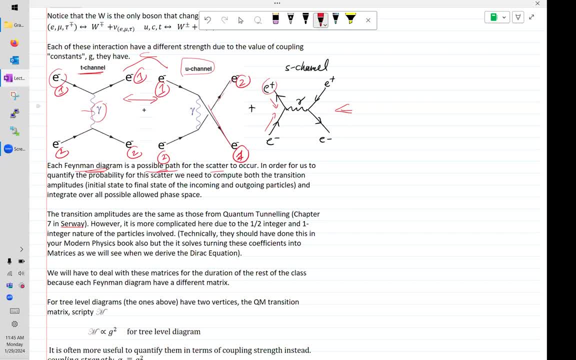 sorry, i still couldn't hear you. you superimpose. what between them do you add? like their funkiness? what was it called? that's what they are: imaginary numbers. anyone on zoom, remember what do you add between them? okay, so, since we're anyone on zoom, actually. 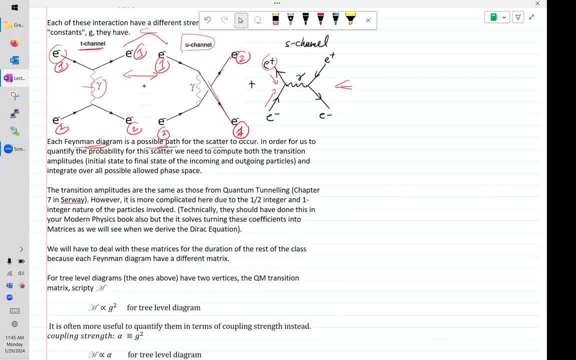 might be interesting to here zoom land. are we still up there? sorry, okay. so i think, um, i think i wrote this somewhere down here, but what you add is actually their amplitude, okay, and it's actually the amplitude square that gives you the probability of that process happening. so let's say, i have this t-channel process, right, right, so this, this has. 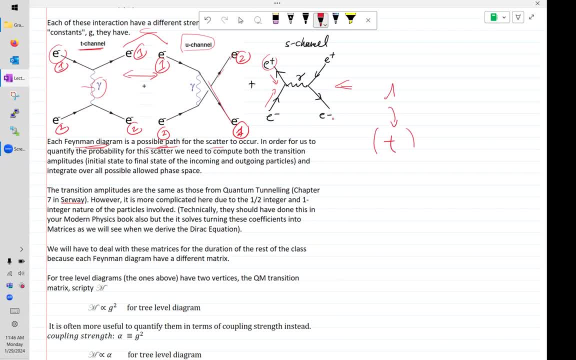 some numbers or something, and then this, and then you add the amplitude. okay, and so that's what we're doing. and if you scale that, scale up, and we have, like this, this mega square right here, and then that's associated with it, so okay, so this has some amplitude associated with it. amplitude okay. 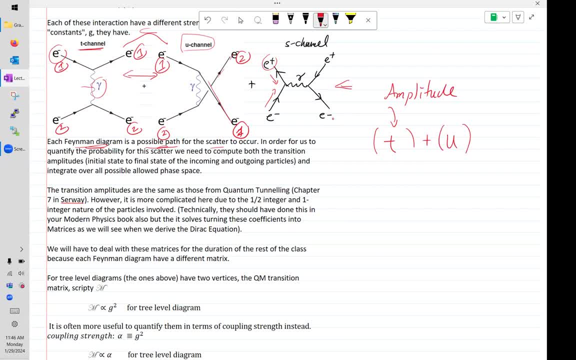 and then the u-channel has some amplitude associated with it. okay, since you cannot tell it's a t-channel or the u-channel, okay, what you do is you basically square both of these together, so they could- I think you guys were trying to talk- say this: they were they. 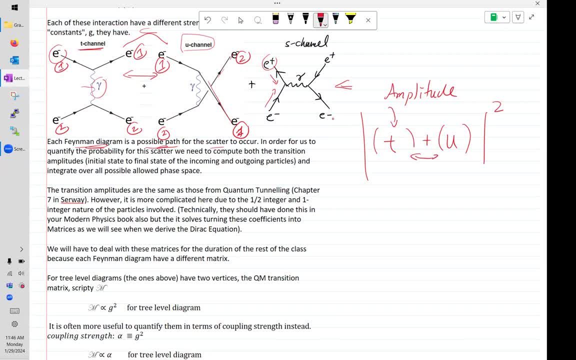 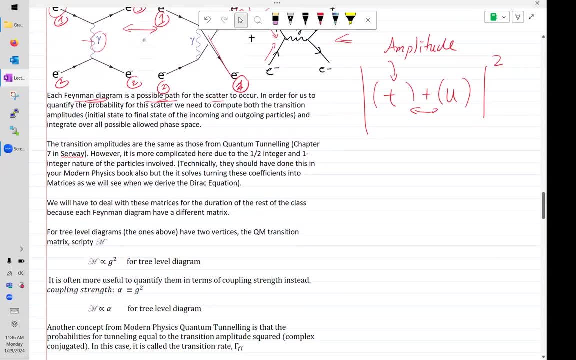 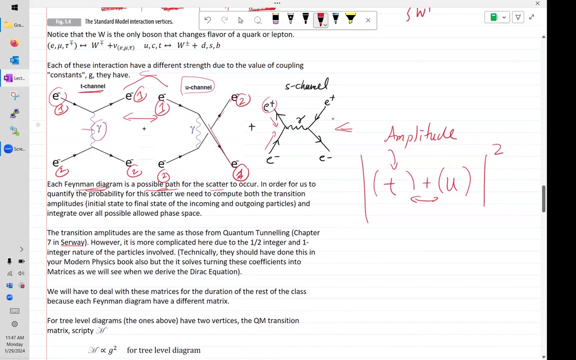 were, could constructively or destructively interfere with each other, depending on the phase between them. okay, all right. okay, so that's how? Yes, quick question: what is the significance of e-channel versus u-channel versus s-channel? um, they are physically different, right? so one of them has an electron coming in, the same electron coming out. right, um, the electron. 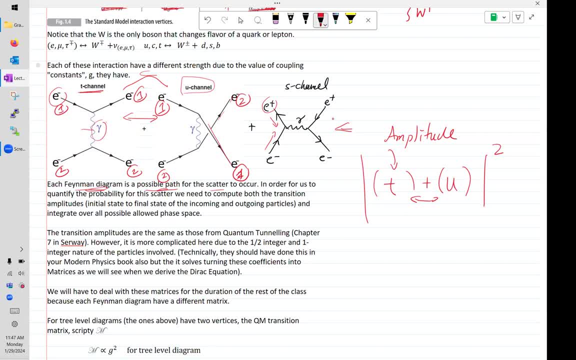 one goes in, electron one goes out. electron two goes in. electron three goes in. electron one goes up, um, go up north, i guess, go upward right, and then the second one, you have the second electron going downward. and but but if electron two was to cross path, electron one- and this is 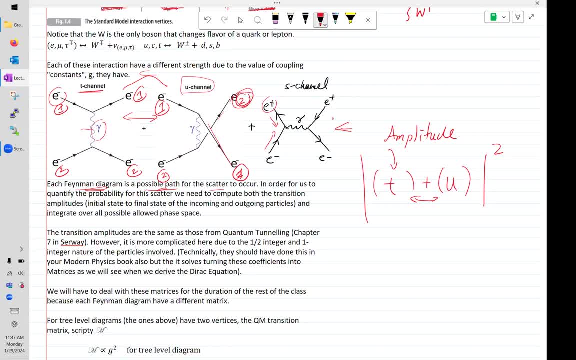 actually a different particle right that came out on the top right. it is a completely different. if you have you as if you cross path and then imagine, like you know, you have like a twin brother or something like that, you can play this trick right where you cannot tell the difference between the. 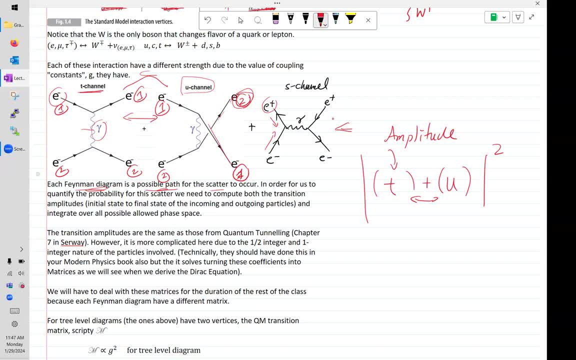 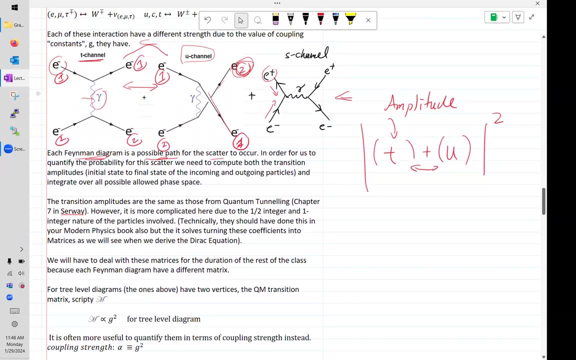 two. so but if, if this case, if down here is like a muon or something and you can tell the difference between them, then you would not have this, uh, quantum interference process. okay, so in t channel do do they always have it where the, the particle on the top, stays on the top. yeah, you chant, yeah. 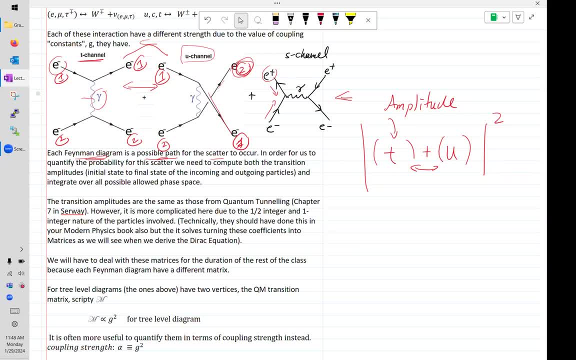 they swap, then the s channel does some sort of other annihilation, which which you know it can't be the same particles, because they won't annihilate. yeah, gotcha. okay, you might um professor too. i know we're almost out of time, but do you mind if i 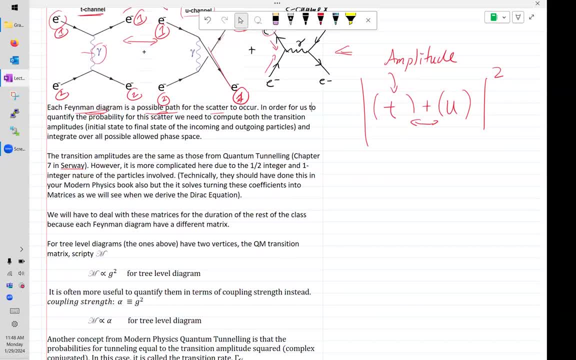 interject a couple things. yeah, just quick. um, i just want to say, because i know at sonoma state in our modern physics classes i don't even know if they use the terminology of amplitudes, like i think we don't really learn about that- tell real quantum mechanics.